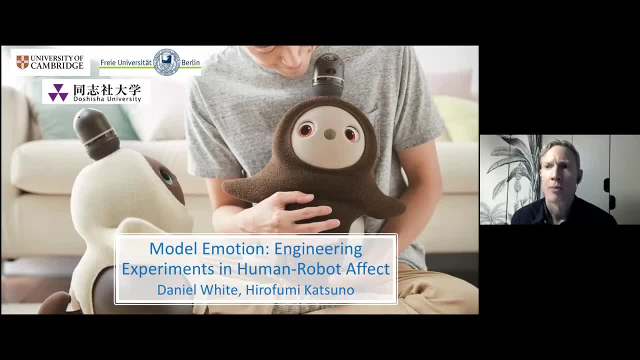 context and detail as I can, But I think this format might help set us up for some productive discussion later. And I'm trying to narrow the question because obviously there are a lot of interesting philosophical questions that could be asked about emotions- and about machine emotion for sure- Ethical questions about whether we even should build robots with. 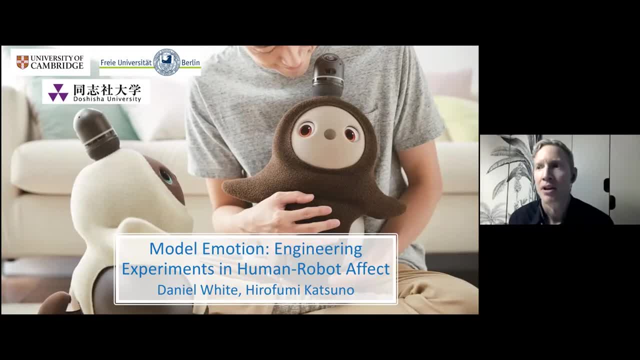 some kind of artificial emotional intelligence, And we can definitely go down that road in Q&A if you like as well. But what seems kind of of most value to this group here, as far as I sort of understand where people are coming from, is perhaps the thing that Dr White and Dr White are. 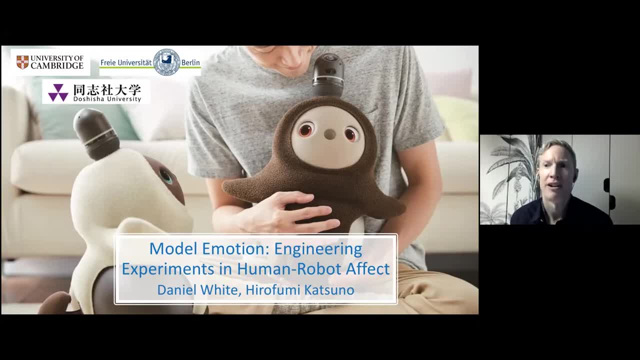 talking about, which is the idea that we can build robots with some kind of artificial emotional intelligence, Perhaps to think of how to build cross-disciplinary dialogue between the human and hard sciences, Because that dialogue itself is- I think many would agree here- important and can. 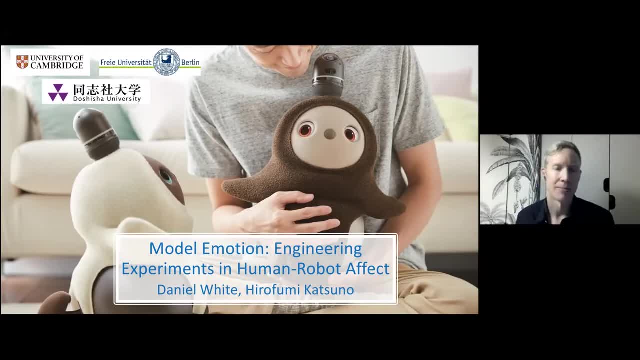 be used for different ends. So we can kind of sidestep some of the sort of philosophical questions in order to sort of get to the practicality of how those questions are often exercised and implemented in research, design. And again this is. I think we can start here, because 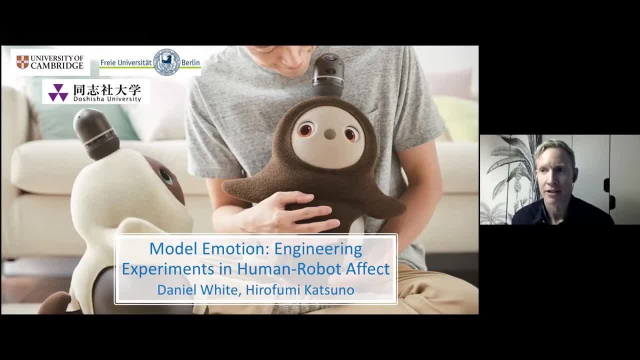 this will be a question for the final part of the panel in the Q&A, So we can kind of sidestep some of the sort of philosophical questions in order to sort of get to the practicality of how these questions are implemented in research, design. And again, this is I think we can start here, because this will be 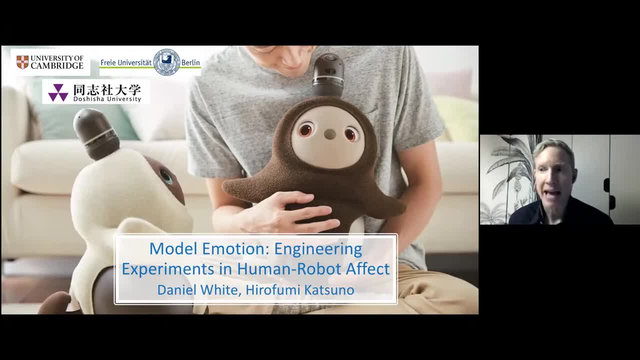 a question for the final part of the panel in the Q&A. So I'm just going to give you a couple of slides and then we'll go over some of the things And then I'll just add a couple of things so that you can get to the point that I would like to add to that. But I'm going to stop there. 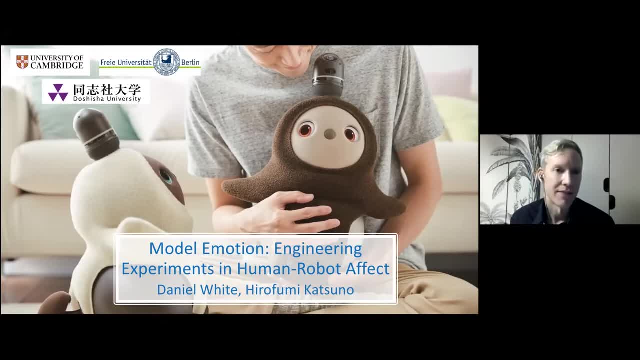 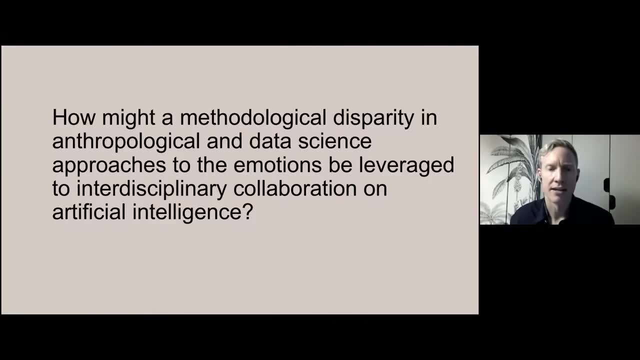 So I have a couple of slides here and then I will pass it over to the panelists. Thank you, Thank you everyone, And this is a question I want to ask you about this question, because it's actually a really phrasing this question in a more kind of academic way, is to ask: how might a methodological disparity 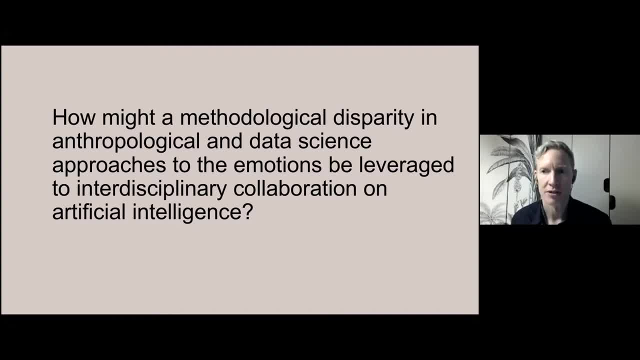 in anthropological and data science approaches to the emotions be leveraged to the to interdisciplinary collaboration on artificial intelligence. so to address this i want to do a number of things. first i'll present what i think is kind of one of the dominant approaches to modeling emotion in machines from the data science perspective, particularly in japan. then i'm going. 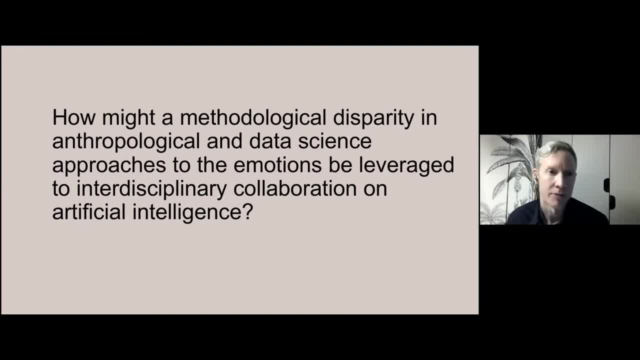 to try to contrast that briefly with how an anthropological perspective is a little bit different. then i'll draw on a couple field work examples of some social robot users and some makers in japan that illustrate some of the experimental and interactive ways that emotion is produced in particular contexts over others, and then i'll try to use those examples to explain why. 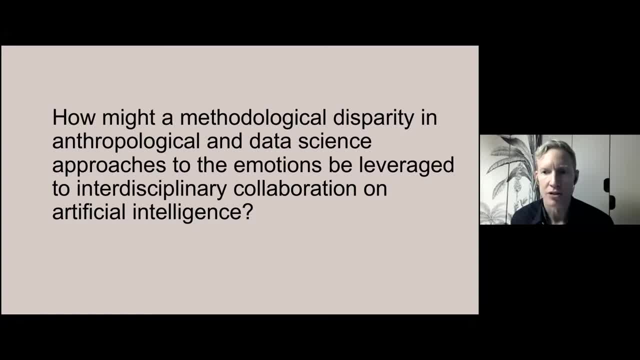 my research collaborators and i adopt some of the approaches we do to constructing dialogue between anthropologists and engineers on modeling emotion, and this modeling emotion is kind of a key word for us and i'll return to it in a moment and because i'll be drawing on examples from japan, i'm aiming 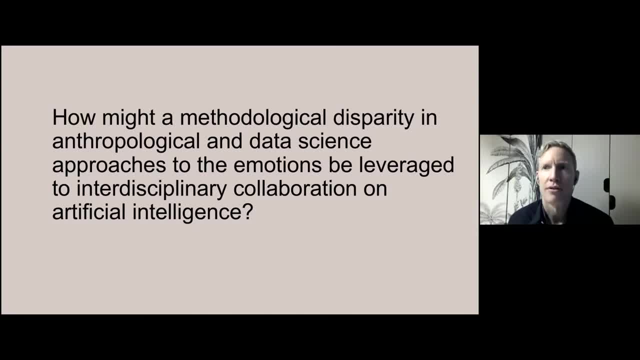 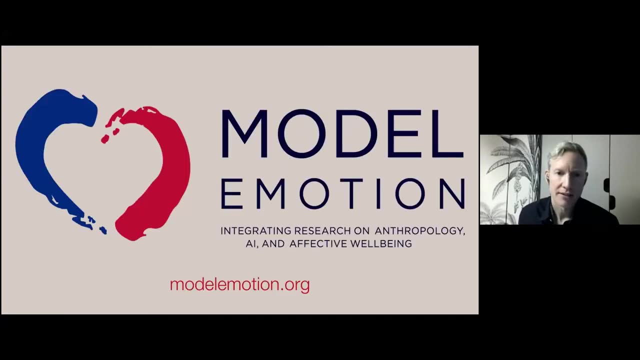 to kind of infuse this whole talk with the question of socio-cultural diversity, in terms of how emotions are theorized, how they are translated into machine viable systems and then how they impact in human robot machine settings. so, like i said, our project is called model emotion and this work comes out of a four-year project that i've been conducting. 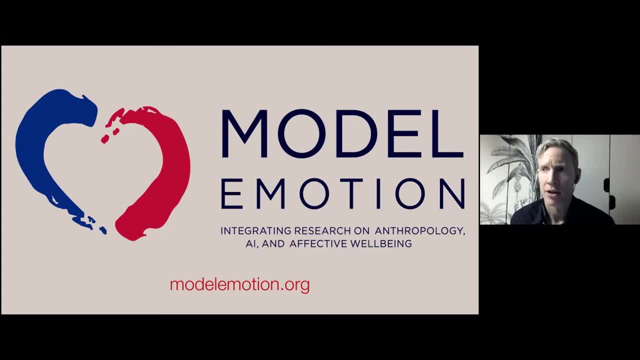 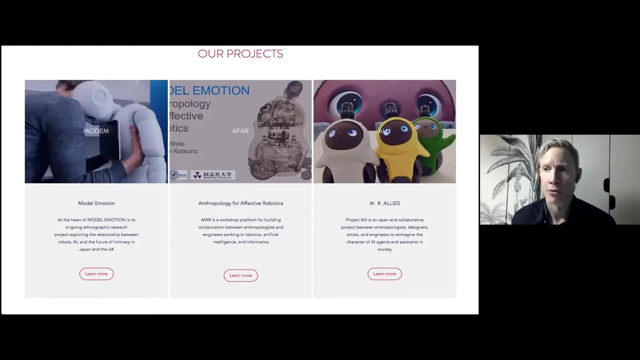 with a colleague of mine, hirofumi katsuno, and this is why i'll often use the pronoun we in the conversation today. so model emotion is this four-year project. it has an emphasis on the idea of emotion and how that emotion is interpreted and how it's implemented. 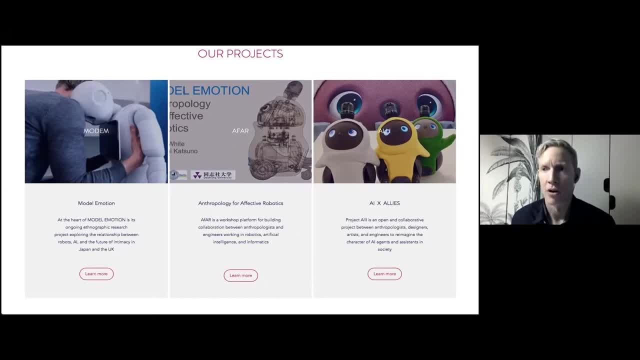 and how it's interpreted in a way that is inclusive and that can be used in a variety of different ways. so it's based on a number of different elements, including your field work among robot producers in japan, as well as some field work here in the uk, where we both are at the moment. 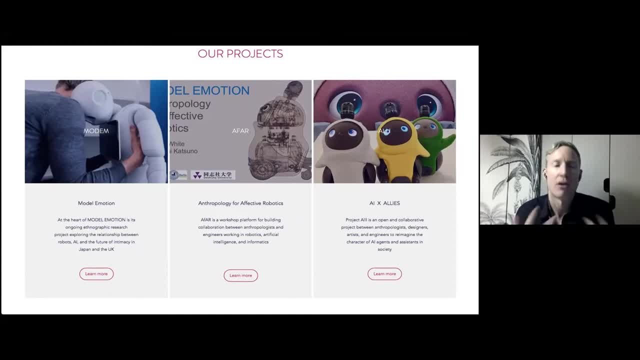 and in both of these sites we attempt to look at how engineers build models of emotion to replicate in machine systems, whether software programs that function in robots or hardware. that embodies that we might say Why we choose this phrase: model emotion. I think this will help explain the 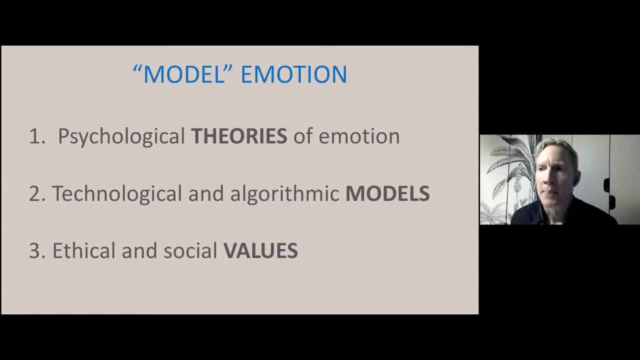 perspective I'm coming from quite a bit is because we think this word model nicely captures the interconnected theoretical, technological and then both the social and ethical dimensions of scientific practices when it comes to modeling emotion in machines. So on the theoretical side, we're interested in looking at how engineers translate psychological models or theories. 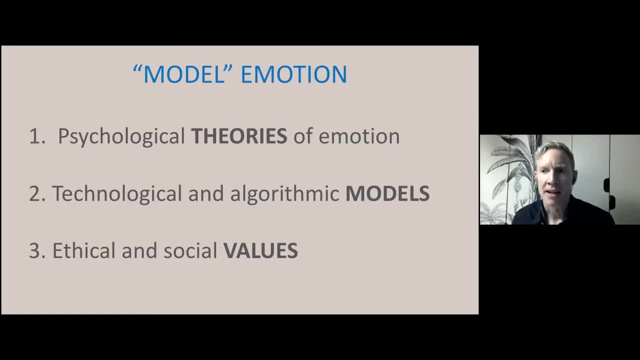 of emotion into machine systems. Then, as a technological practice, we want to look at how those theoretical models are translated into machine systems, whether it be in software or algorithms used to generate emotional data or read emotional data, And then we want to look at it as 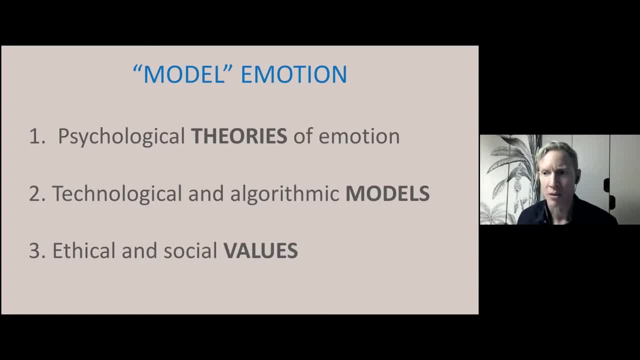 a social practice, looking at specifically what happens when you take those machine models and put them into laboratory context or public performance settings, where now those models are doing something in social space and creating different reactions, creating different data. that has to be taken into account, in fact. 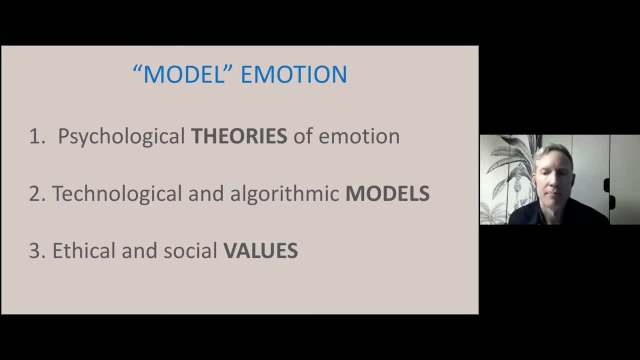 And then of course, there's all kinds of ethical dimensions that are paired with this, referring to what kinds of feelings or emotions are seen by people, by robot users, as valued or coveted or ideal for a society. And that's also kind of one meaning of our quote, unquote: model emotion. 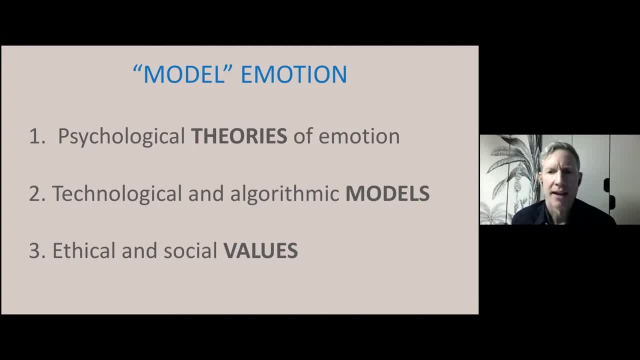 Um, um. so, with that said, I want to maybe start by just coming back to what I think is, um, maybe not necessarily the most popular model of emotion among engineers very recently, but something that represents a basic paradigm in emotion modeling, maybe even more so in Japan than in other places. 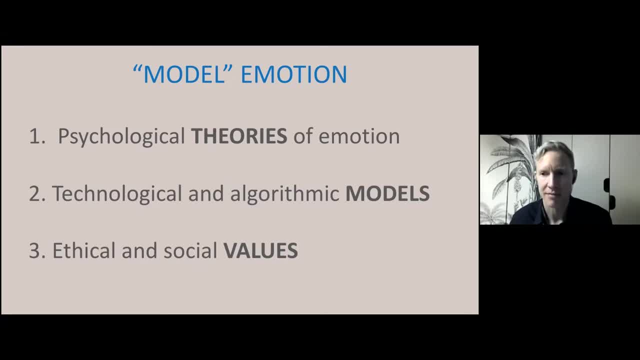 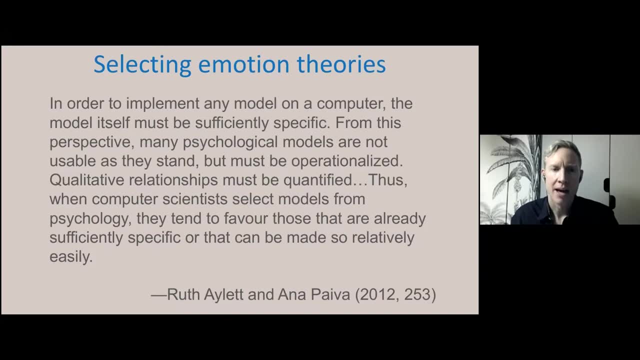 which is very interesting, considering where this model came from, given its history, Um so. So one good example in talking about how emotion models are selected, how emotional theories, often from psychology, are selected for machine inscription, is to turn to um. one good way to approach this is to turn to computer scientists themselves, um, who are obviously, um, quite. 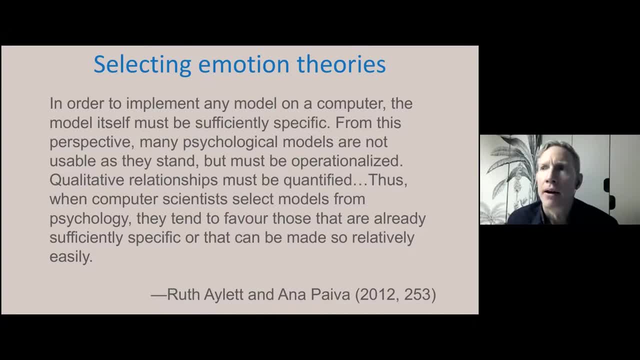 reflexive and reflective about this practice. Um. so as computer scientists Ruth Ailet and Anna Paeva write about emotion recognition systems, Um they say that in order to implement any model on a computer, the model itself must be sufficiently specific. 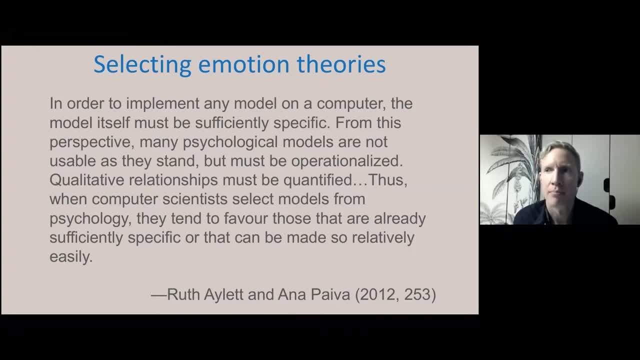 From this perspective, many psychological models are not usable as they stand, but must must be operationalized. Qualitative relationships must be quantified. Thus, when computer scientists select models from psychology, they tend to favor those that are already sufficiently specific or that can be made so relatively easily. 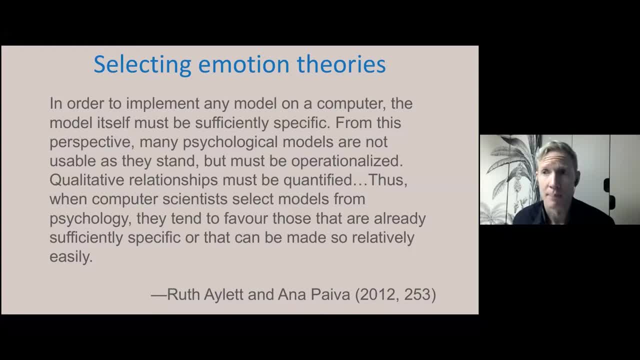 I think they hit the nail On the head here with this description. Um so let me just jump straight to one example from Japan, my first kind of ethnographic vignette that illustrates this problem quite nicely. So this is powder or power. 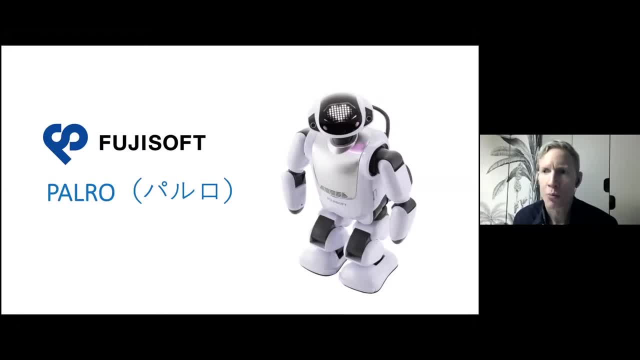 Um, this is a small, uh humanoid robot created by the software company Fujisoft in Japan, And powder was created specifically as a communication partner for the elderly. So it's engineers. Imagine that Pardon you Leave the loneliness of, for example, aging parents in Japan, of which there there are many. 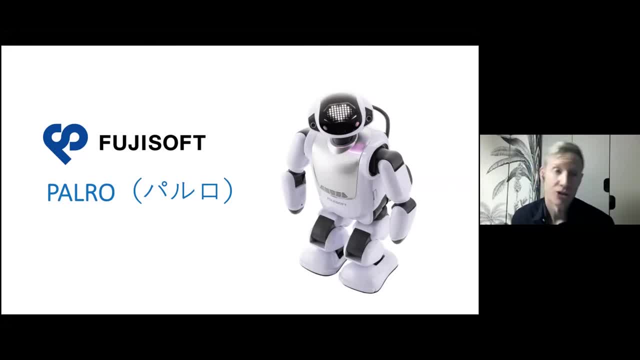 Um, as well as relieving the anxiety of their children, who worry that they can provide them with care that's traditionally expected of them. So powder can carry on a basic conversation and is designed to hold the user's attention and interest. And, of course, integral to this objective is equipping powder with some emotional capacity, some capacity to read the effect of state of the user's аtysm. 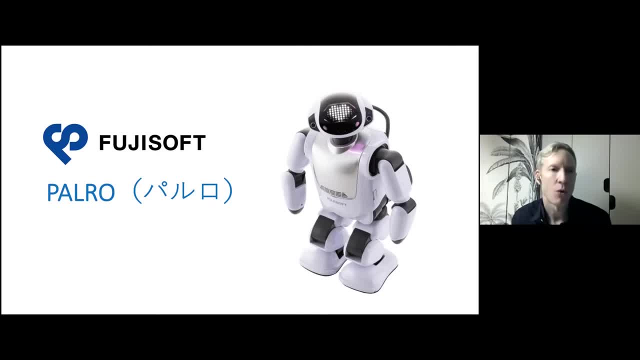 And, of course, integral to the subjective is equipping powder with some emotional capacity, some capacity to read the affective state of the user. Um, but also- and I'm not saying I don't share this idea here, But I think that is a very interesting perspective. 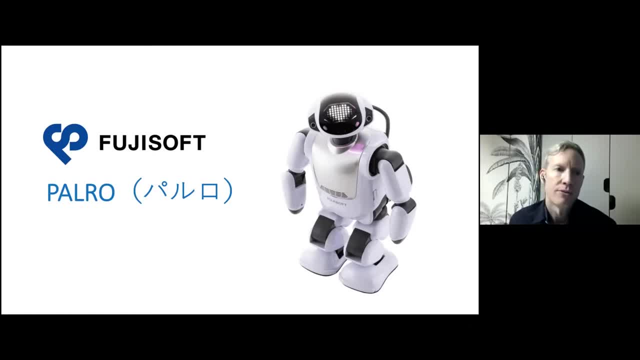 So this is皆さん's perspective and you can definitely go back to it user. So if Parudo, according to Fujisoft representatives, can sense when a user is becoming uneasy or unengaged in interaction, the robot can better learn how to adjust the content. 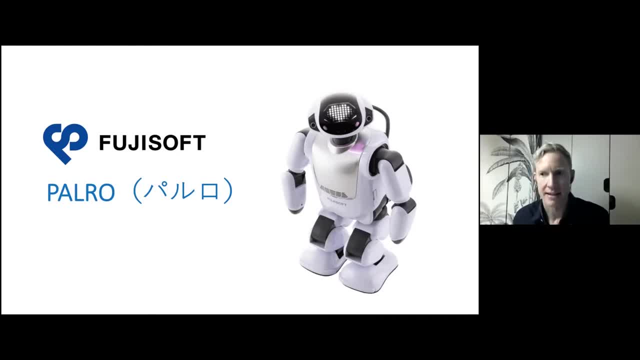 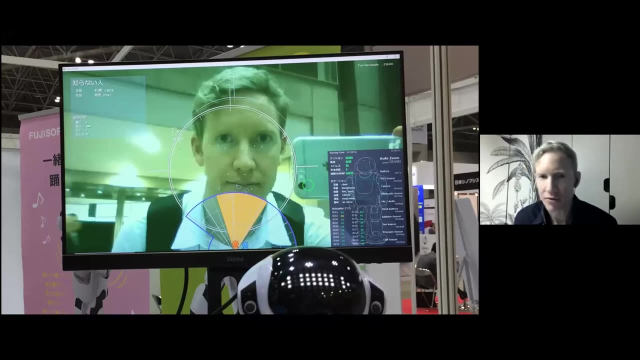 of conversation, or perhaps suggest an alternative form of entertainment, such as singing a song or performing a dance or something like this. And then this is how Parudo reads quote-unquote, or senses emotion. So in this photo, Parudo is reading my own face and, more importantly, my. 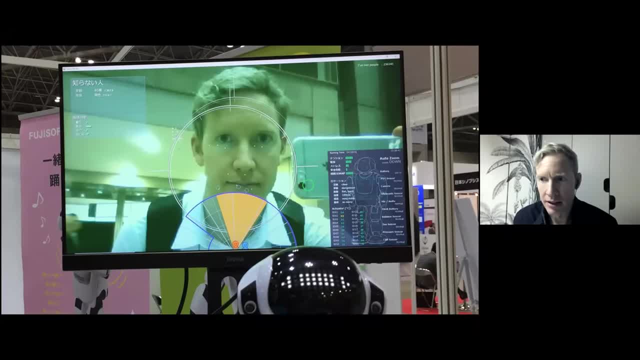 own facial expressions, And in the top left corner of the screen should be the left in your sign as well, although it's probably a bit hard to see there. but there are listed these kind of four emotion labels and then different quantities to what degree that emotion is being expressed. 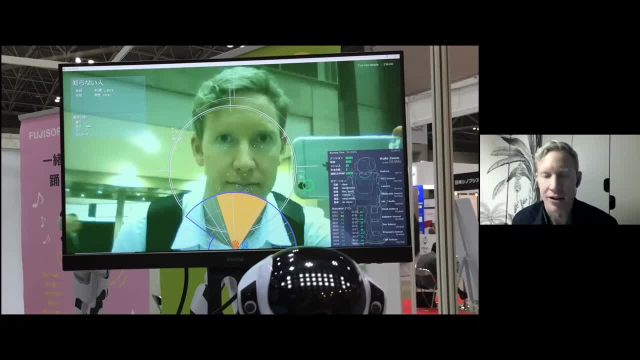 And these would translate as happiness, surprise, anger and sadness. So this is how Parudo's algorithm, quote-unquote, sees the emotional world, And this is what I call, as an analytical term, a quote-unquote model emotion. It's modeled because it has this technological system, obviously. 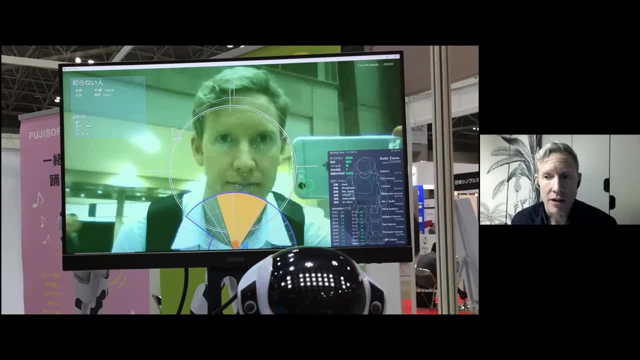 at work here, And it's modeled because it's drawing from a specific psychological theory or model of emotion, And it's modeled because it has this technological system obviously at work here in order to instrumentalize it. um, so this is probably the part of the talk that i think a 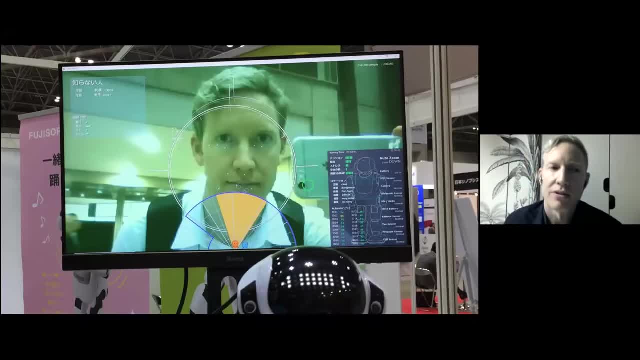 lot of you will know about, but for those who don't, i just want to touch on it because it's it's quite interesting, specifically when placed in the context of japan, where these psychological models of emotion are being taken up so interestingly enough. the model of emotion. 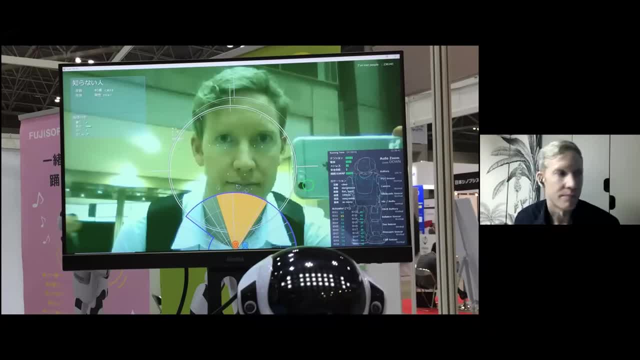 that powder uses, like many um social robots in japan these days, or at least the place that they start is with paul ekman's model of the basic emotions. again, i think you've likely heard this before, but, like, let me go through it a bit and just contextualize it. so, um, here's paul eckman's 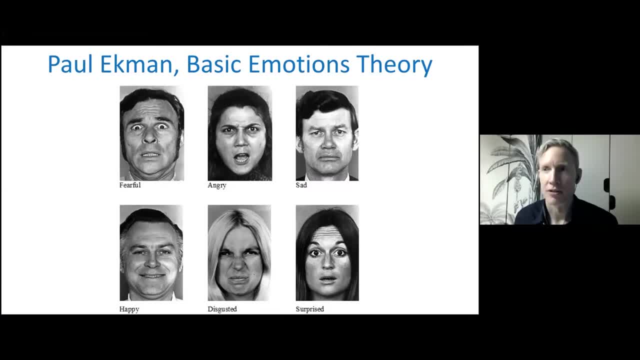 work. you know, over 40 years of research on the expressions of the emotions um, beginning most prominently in the in the 70s. the american psychologist paul eckman here developed- and that is, i believe, that's his face in the top left, actually developed- a model of six basic emotions. 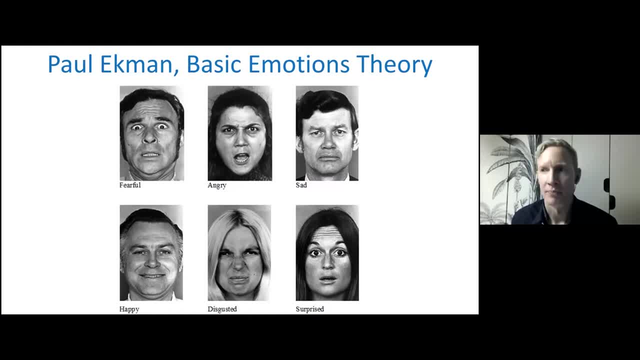 sometimes it was described as nine, um, often now it's described as seven, but either way, he considered these kind of universally identifiable emotions, which can be seen in facial expressions across cultures, even more important than his theory of basic emotions. was this, this coding system in which um these emotions were rendered? 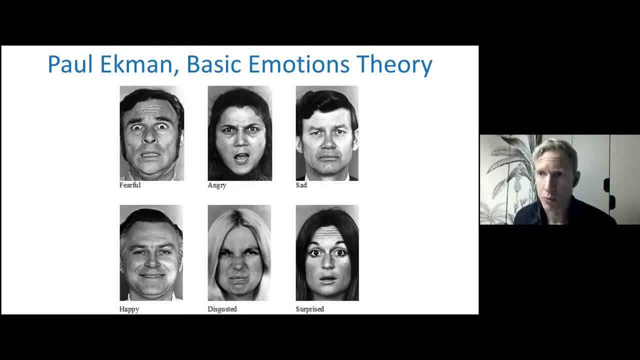 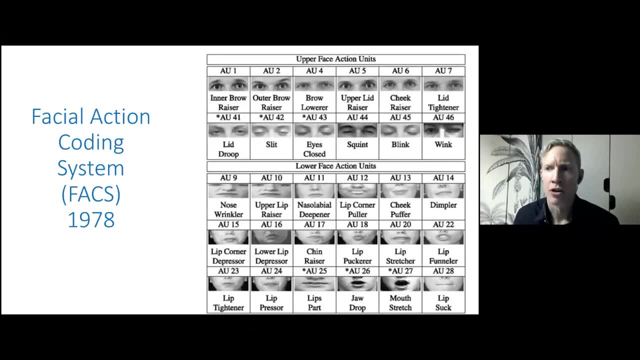 understandable or interpretable. so, in conjunction with wallace freeson, and then drawing on the work of the anatomist called hermann hiltz, eckman designed what you might know is the facial action coding system, or fax, and then using facial action units measuring minute or micro movements of the face, 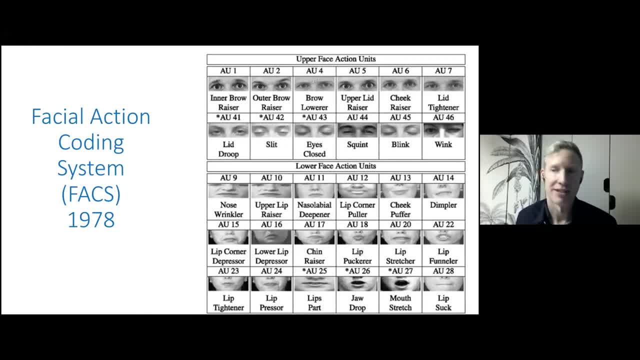 some of them arguably automatic and non-conscious, which is a super interesting dimension of this. fax provides this integrated and systematic means to code facial expression in a way recordable and programmable then very easily in software. um, and when i say easily, i mean it's codable easily, not necessarily that it's easy to 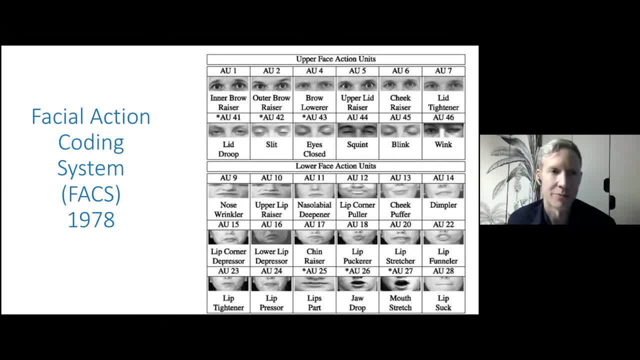 understand what kind of emotions you are coding, which is kind of the crux of the problem we'll return to in a minute. so with this um coding system it becomes then very much. so eckman's model of the emotions more generally has become the fundamental basis for 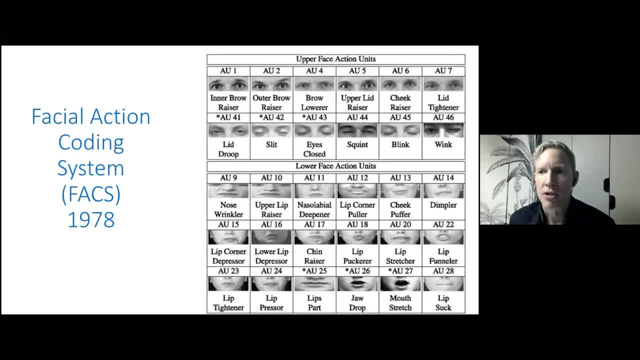 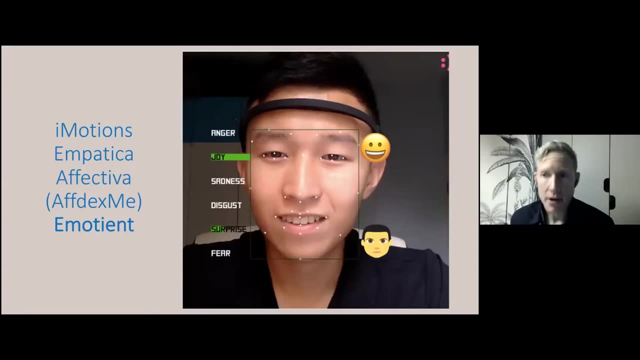 starting out and experimenting with machine systems, um or robots, and giving them a preliminary form of artificial emotional intelligence. so today there are several companies in north america and europe that employ or build on this original model of emotion, creating affect sensing technologies, including affectiva, i, motions or 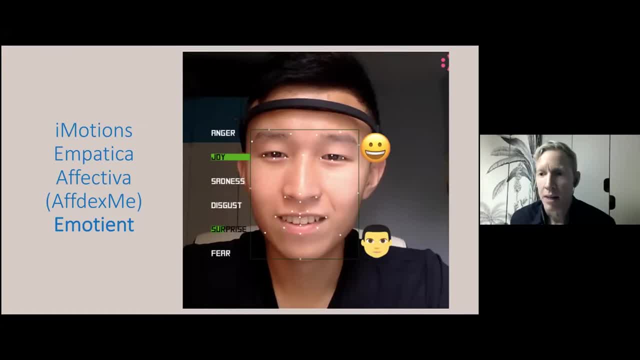 the company emotion, which no longer exists, but was a company that, in fact, eckman served in some consulting capacity until this company was bought by apple to basically provide the facial recognition technology that unlocks all of our iphones today, and it's still, to this day, eckman's model that is actually most dominant in social robot engineering. 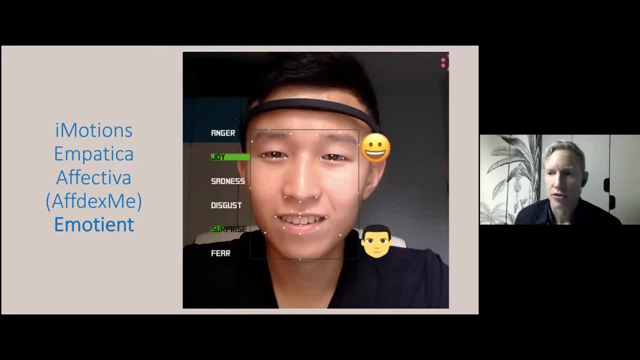 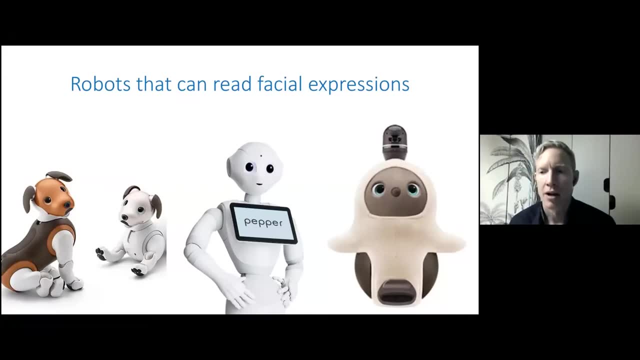 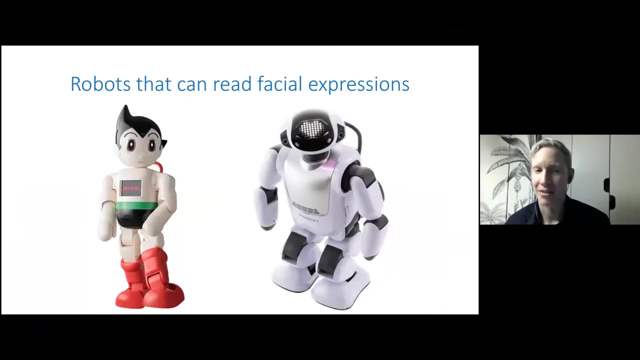 in japan. um, and here are just some of the mass marketed companion robots using this model in japan today in one sense or another. some of these robots can read facial expressions, but don't often but have the capacity to, or are sort of ready to be updated in the next software patch or update, and some of these robots actually 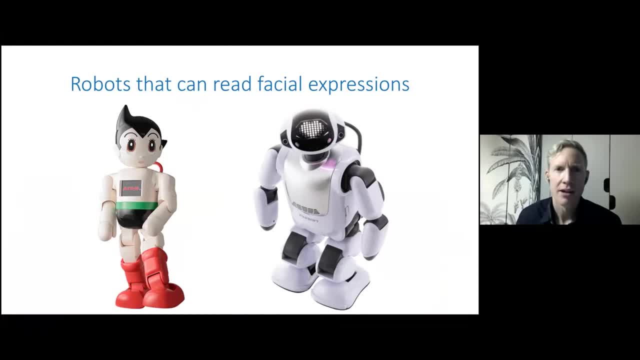 do incorporate a version of that model already, Okay. so I understand very well that there may be some engineers and computer scientists in the crowd who say, yeah, we all know this. Ekman's model is a very simple and basic model and we understand emotions are far more. 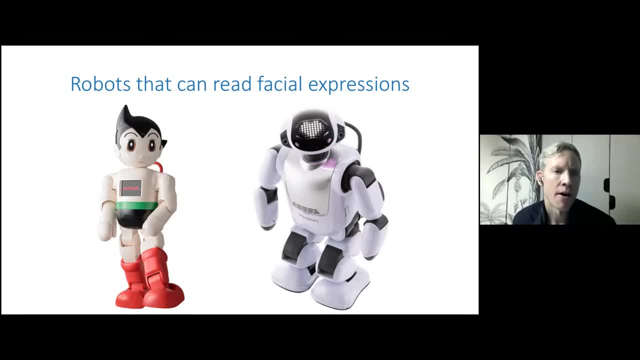 complex than that, and yet for many of the mass produced social robots in Japan, they very much still do rely on this paradigm of what the emotions are, namely a kind of feeling category that can be sensed and understood quite similar, similarly, if not universally, across all cultures. and that's of course an interesting point to take up for an anthropologist, a cultural 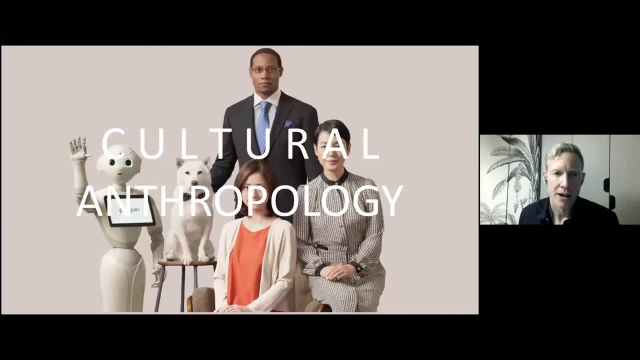 anthropologist like myself, I probably don't need to take a lot of time raising the kind of anthropological challenge to this universal model of the emotions, especially to this group. but let me just briefly state that even very early in the formation of cultural anthropology, especially in what later came to be called the culture and personality, 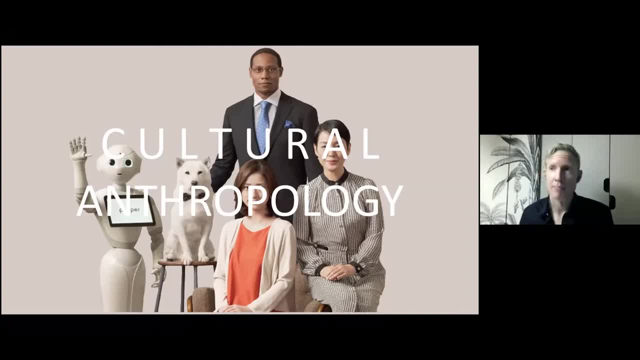 school in North American anthropology which was associated by people whose names you've heard before, probably like Ruth Benedict and Margaret Mead. Ruth Benedict's early work was actually on Japan, or at least some of her work was on Japan, and it was a work which very much characterized. 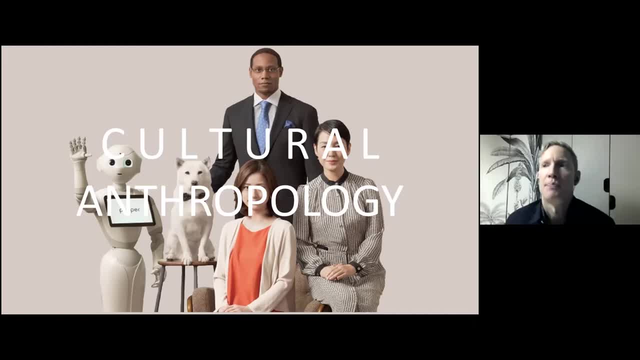 the cultural and social interactions in terms of emotional differences, which is very interesting to take a look at. So very early in anthropology, emotion was actually quite a prominent topic, not just of interest in general but as a topic through which to discern cultural variability. So this question has been with anthropology for a long time. This perspective was asserted even. 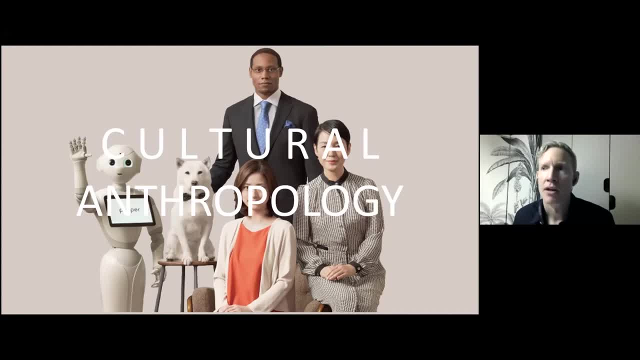 more strongly in the 1970s and 80s, when anthropologists started studying the this emotional diversity most explicitly In what was called the, what came to be called later the anthropologist of emotion, and here mostly anthropologists were looking at how certain emotion labels 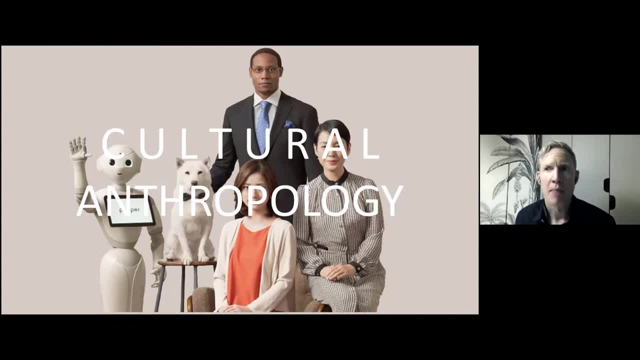 in english, like fear, for example, did not always map onto neatly corresponding categories in other cultural contexts. what you call fear in english is not the same thing that you might call ikari in japanese. um, sorry, that's, did i say anger, anger ikari, or something like fear, or kyofu in japanese. 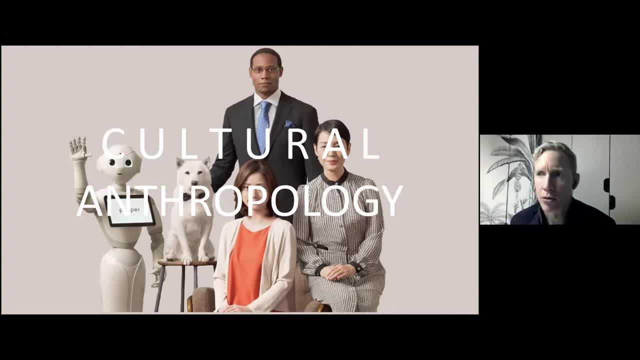 so this work on the diversity of emotion continues today with anthropological and humanities work. um, there's really, you know, emotion and affect is quite a popular topic across both the human and hard sciences these days. for other interesting reasons we could go into um and sometimes um. this emotion work today in anthropology focuses on what scholars call 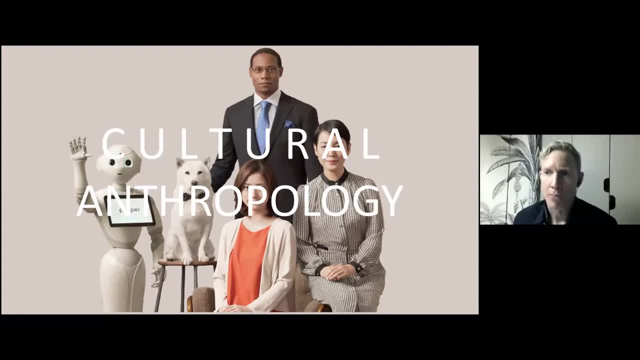 affect or affect theory, and one main contribution of this um kind of new terminology is to try to point to the cultural diversity not only of signaling processes of emotion, in other words how feelings are expressed in words or facial expressions, um stories and symbols, but also in how feelings are experienced somatically and 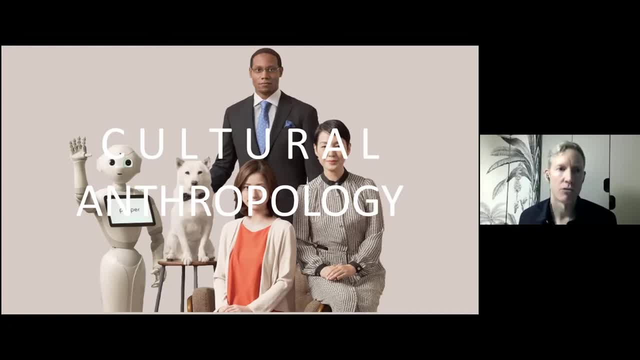 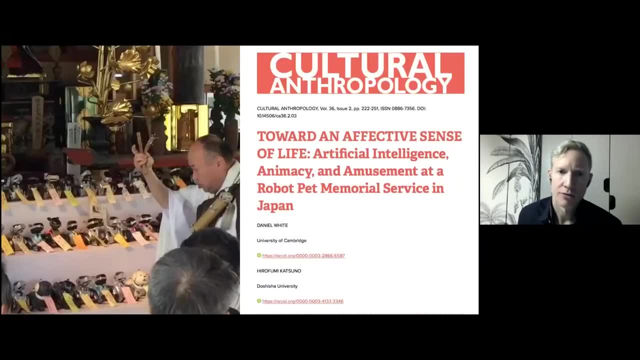 physically in the body, that can also have a very cultural dimension. um so, my colleague hiro, um so fumi and i very much see our own work as contributing to this aspect of anthropology. um so, for example, we have a recent article out on robot funerary services. um buddhist. 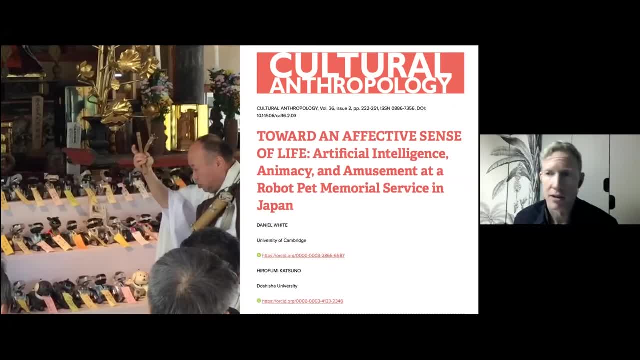 robot funerary services for for robots in japan, where we see some very interesting ways that people use robots in order to actually facilitate a kind of emotional interaction with people, in the sense of of losing a, an artificial pet which is. it's quite an emotional experience in some way. 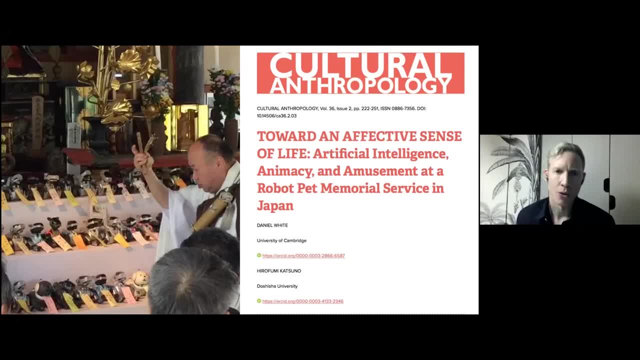 um, and so it's just one example, i won't go into today just because it is out there, but it's one example, uh, finally, i'll just say, in terms of this section of my talk talking about the anthropological critique of the basic emotions paradigm, i'll just say that probably the strongest 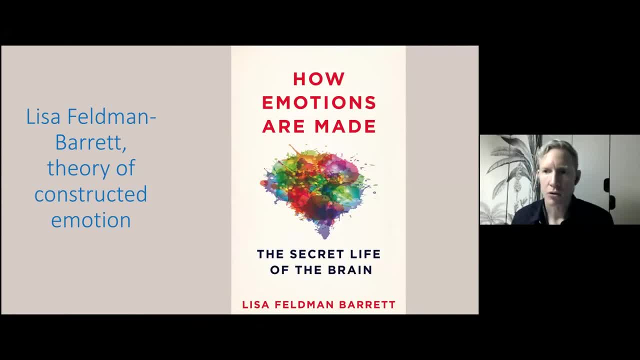 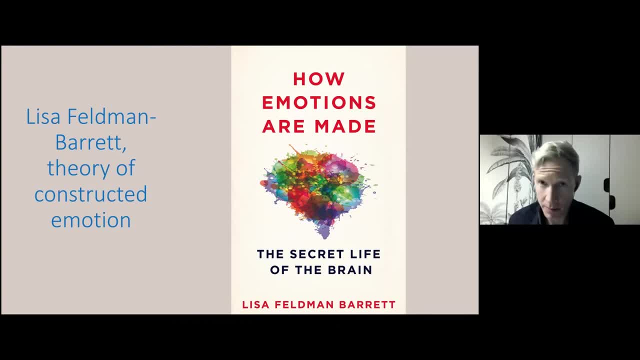 like lisa feldman barrett and this very popular work how emotions are made. so in her constructivist theory of emotion she emphasizes that one really cannot know in the face, or even often in bodily gestures, or even in our eye scans, or neurological fingerprints, as she calls it, or any other of the 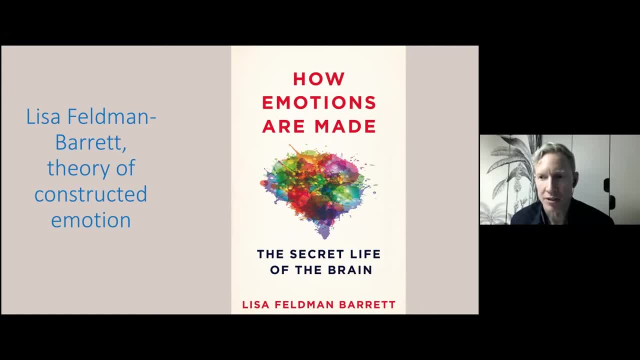 social signaling indicators that engineers often use to build emotion systems for reading and performing emotion. you cannot know from those social signaling systems what people actually feel on the inside of the brain, and so i think that's a really important point that we need to think about. um, in fact, people themselves. there's often this gap and a kind of affect emotion gap, as i sometimes 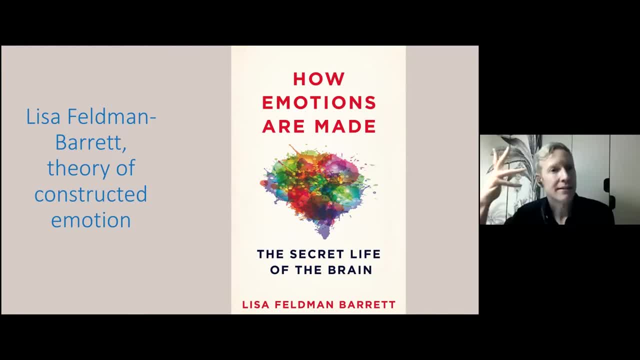 like to call it, between how people are representing um emotions or feelings in their body to themselves and then those feeling states themselves. there's always this sort of epistemological gap there, into which or through which all sorts of interesting and mechanicalized and often political and ethical things can get done. basically, basically. 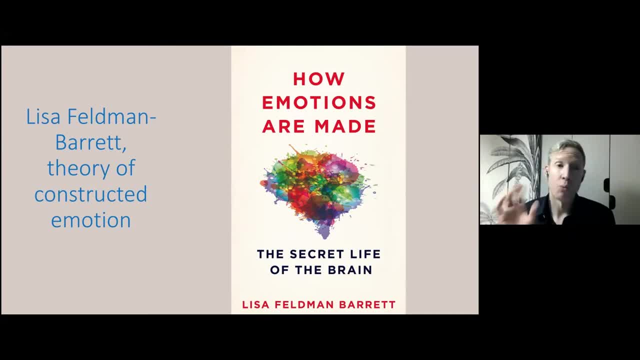 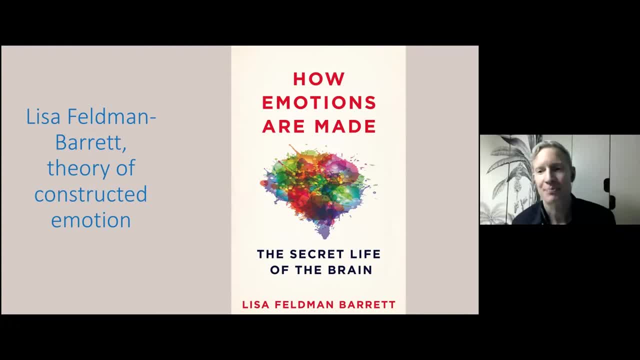 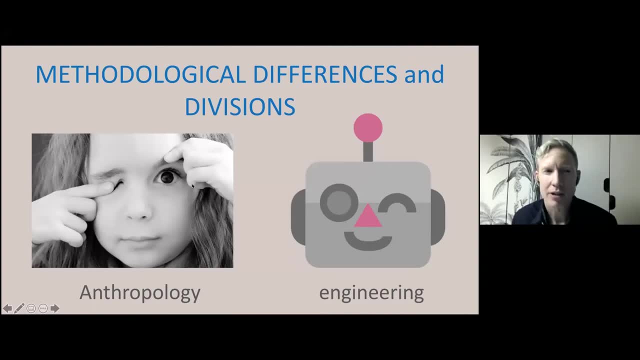 measuring your heart rate. variability might, for example, okay. so my concern about this way of talking, though, about modeling emotion, um, from a kind of qualitative versus quantitative point of view, is that i think that's a really important point, and i think that's a really important point, and i think that's a really important point in my view- is that it constructs a bit of an 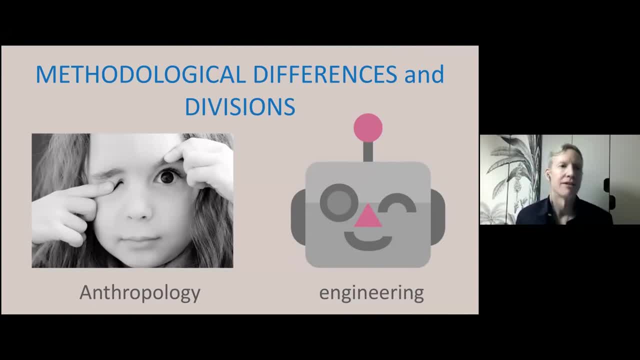 artificial divide between these fields, where we obviously want collaboration, right um. so the prominence of lisa feldman barrett's work has served as an explicit and very public challenge in many ways to artificial emotional intelligence builders and programmers and to the field of effective computing more generally. i think, and this has been constructive in tempering the 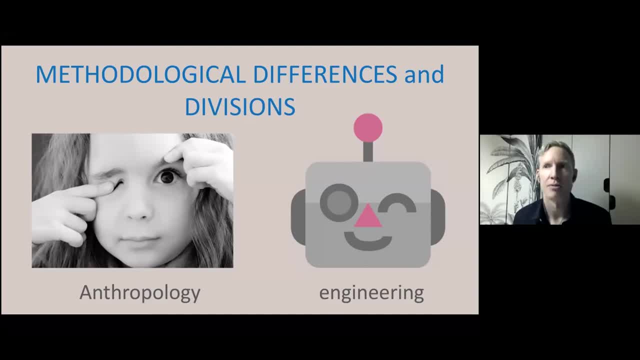 sometimes overly enthusiastic and overstated claims of what emotional ai can do. i think at the same time, my sense from field work among engineers is that it has also created some polarization rather than opportunities for dialogue, where engineers will say something like: well, if psychologists are aren't going to recognize our efforts or anthropologists aren't going to recognize our, 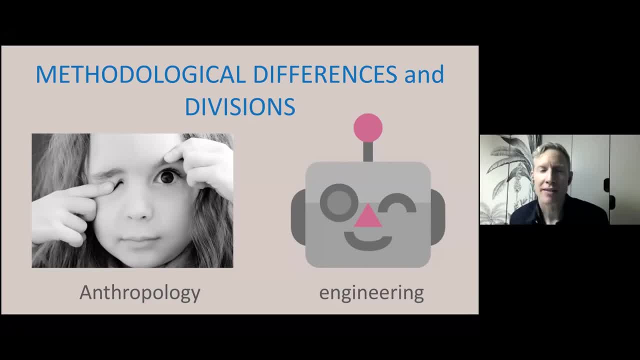 efforts to build better systems. um, knowing that our current systems, like ekman's model, is only one that we are working to get beyond, then we'll just carry on with our own work on our own. because, without worrying too much about these anthropological critiques or social science critiques. because 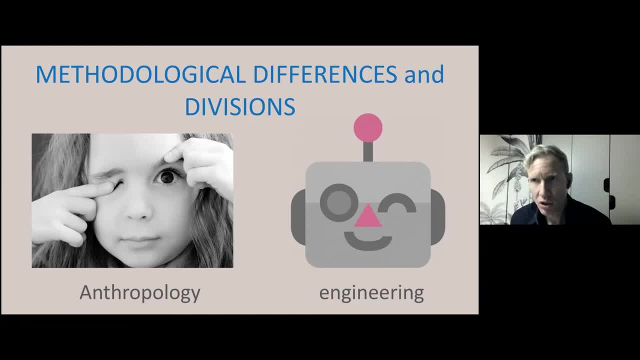 they aren't really being very fair to us. moreover, i think this sort of um binary division between a quantitative and qualitative approach to emotion glosses over the point made clear by many social scientists working on human robot interactions, that many people, for example those um that we 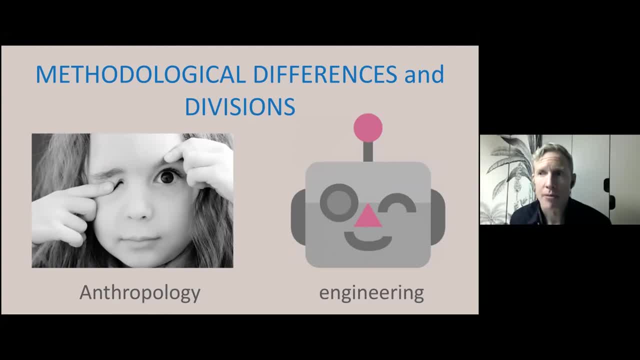 engaged with in japan genuinely welcome opportunities for interacting with robots that have increasingly sophisticated means of responding to humans in either lifelike or emotional ways. so let me take just another quick ethnographic um moment aside here, create a little sidebar just to offer one quick glimpse of some of these human robot experimental contexts in japan. 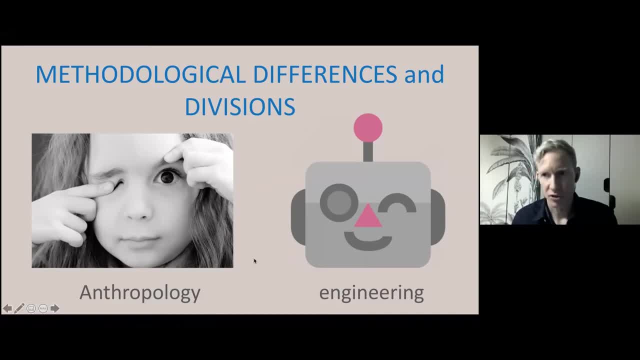 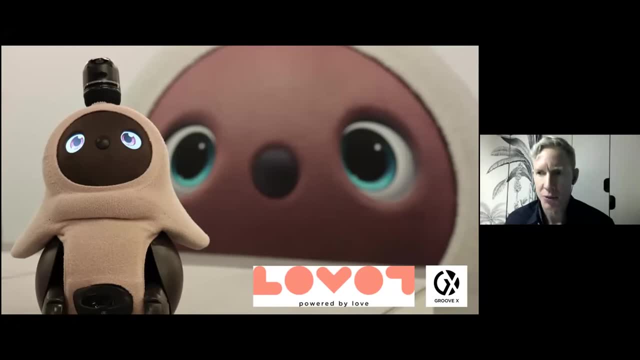 that i'm talking about um. so i'll do this through this robot called uh lava, which i've written a little about, a little bit about um. so i'll do this through this robot called uh lava, which i've written a little bit about. um. so i'll do this through this robot called uh lava, which i've written a little bit about. 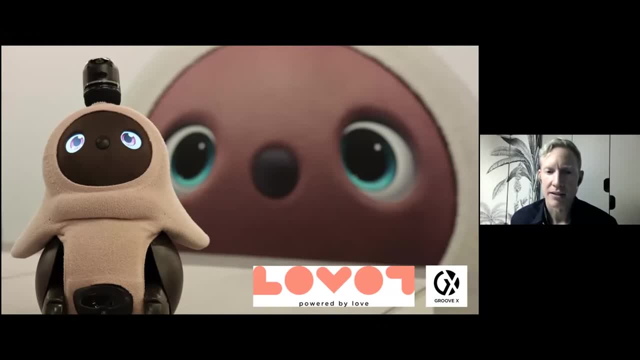 this talk um just before lava was released at um groovex's headquarters, the makers of lava um and there at this event, this talk event, as it was called, i met this woman who i call aya um, and she told me that she's really excited for this future in which humans 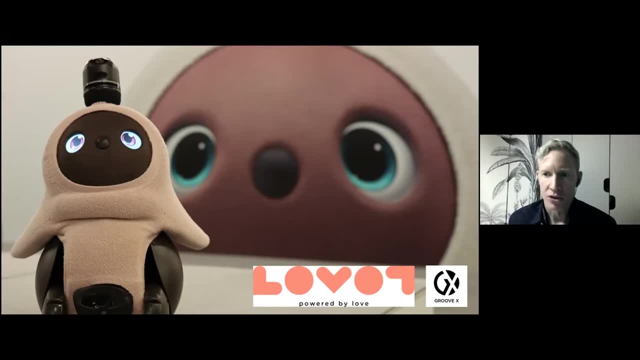 will be able to coexist with robots. so she told me that she didn't think this was possible in her lifetime, or even have much interest in robots at first. but when she learned about lava or raboto, this kind of 40 centimeter tall furry robot on wheels- 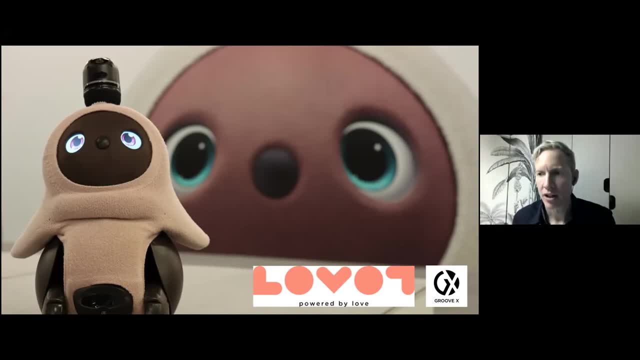 which is designed specifically to seek out and offer affection. she was elated to discover that this future that she had only imagined was now within her reach, seemingly, seemingly so. she urged me to sort of pick up love it while we were talking, because she's really excited about it. 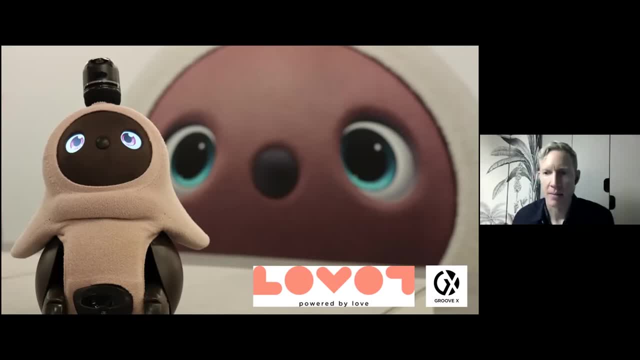 and a few of these creatures were spinning around the table as we were talking. so when i picked up lava, it's really interesting to me because i've been talking about this for a long time and i've got a lot to comment on right. but she talked about workshops we were doing and doing later, right. 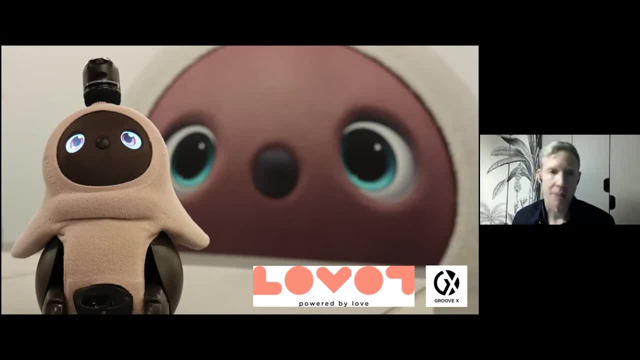 has conflicts, so it's r Drink. when i was holding it, i uh kind of poked its nose which, because it has a sensor in it, elicited something of kind of this irritated giggle from the robot, not a very human-like expression, but kind of a a very animated expression nonetheless. 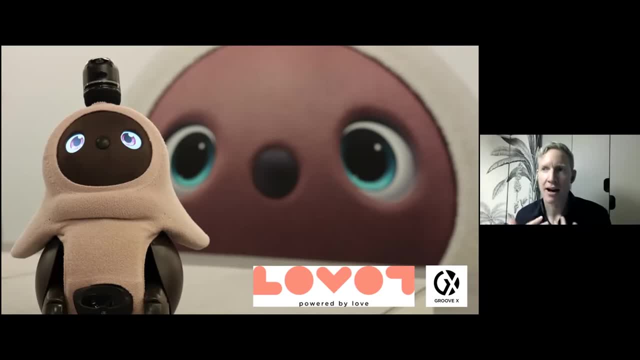 and as we talked, Aya was stroking Cherry's belly and then the robot's eyes blinked a few times and then slowly closed. Aya then exclaimed: oh wow, it fell asleep. how cute or how kawaii. so Aya told me that she was not very interested in robots and technology or anything in the IT. 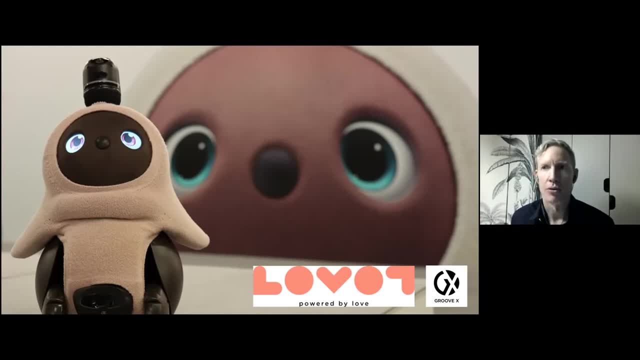 world in general. but when she saw Raboto, she was immediately and, as she says, inexplicably moved by Lava when she first saw it, and she told me that, you know, it's just an emotion, and so the kind of emotion that she's talking about there, this encounter with this new artificial being, is not 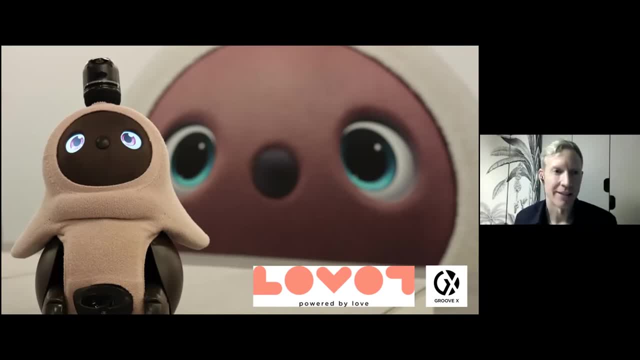 something that is very easily codable. I'd like to propose for engineers these first encounters in human robot affect, we might say. and yet I think both anthropologists and engineers are interested in understanding what that kind of emotional interaction or what that emotional expression and experience is, and how one might code or describe it. and Aya went on to say: 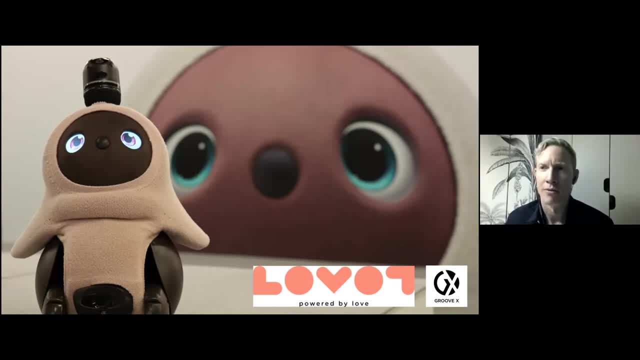 quote: you know about lonely people in Japan right, which is often referred to as Kodoku Nahito in Japan, a kind of a fixed social category, of a phenomenon that's increasing these days with growing elderly populations. so, Aya said, I think that everyone needs to feel affection. 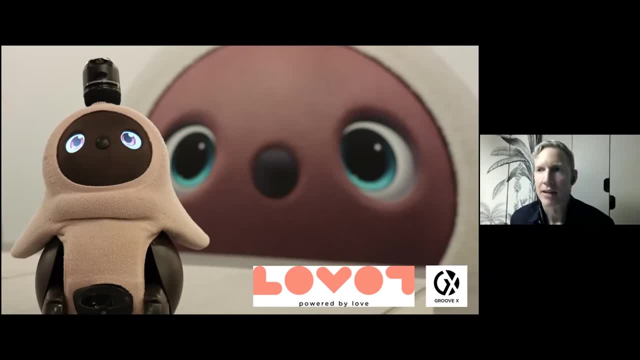 and everyone can enjoy this feeling. we get from cute things like love out here. it fills your heart, but everyone can get this feeling, which is a common theme in Japan as well these days, especially in urban Japan. she goes on to say that I think that in the future, maybe one or two people out of ten 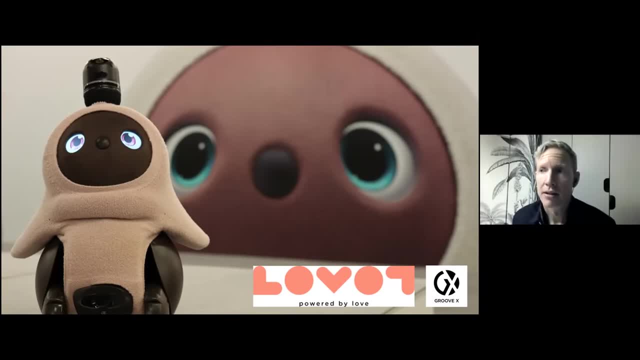 might simply have relationships with things like love art. it's not really any different from the kind of affection one gets from a dog or cat or even another person, and it's their choice. this is a really interesting future. ending the quote from Aya here. so Groovex are really Groovex. 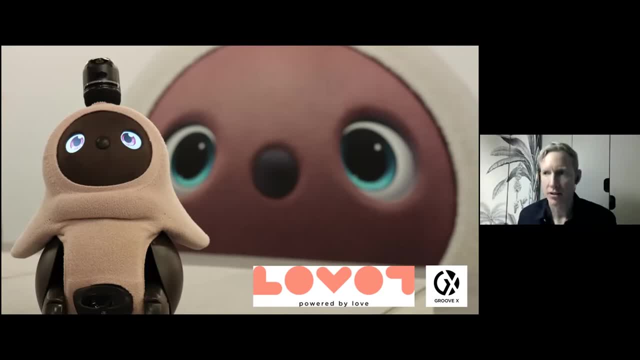 employees are really happy to kind of discover and talk sessions like this and getting a lot of feedback from people like Aya that their efforts to build a robot that appeals to more than just technophiles is paying off. their new robot, Raboto, here again is furry. it roams around the house on. 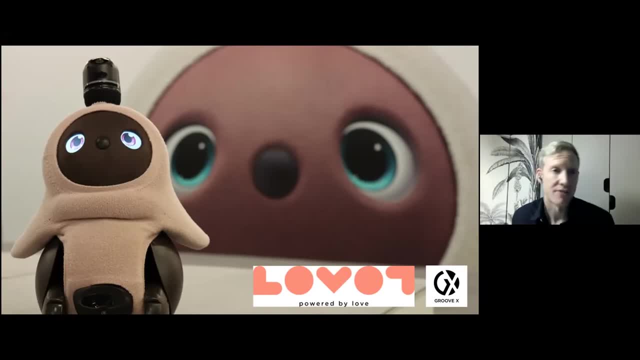 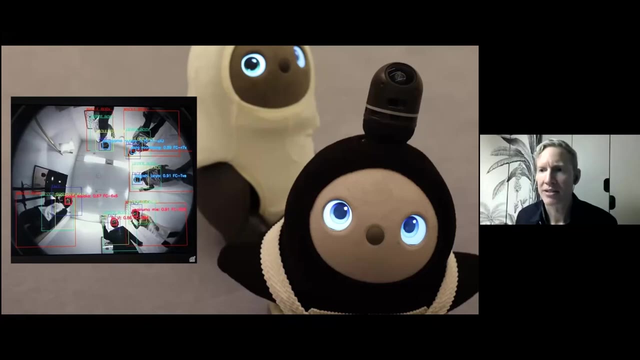 wheels and is designed by the company for the sole purpose, as its founder, Hayashi Kaname, to be loved by you. it has 360 degree mapping on its head, which can, or in its horn, which can map your home surroundings. it has over 40 sensors in its body to register human robot interaction. it has a mobile 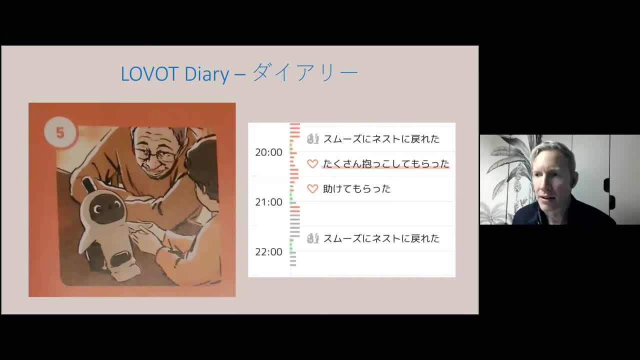 diary system that pre provides this very interesting data set of kind of human robot intimacy that can use by consumers and obviously also used by the company as well, in order to code human robot emotional experiences in a different way than you would code. just a facial expression, right? so this is. 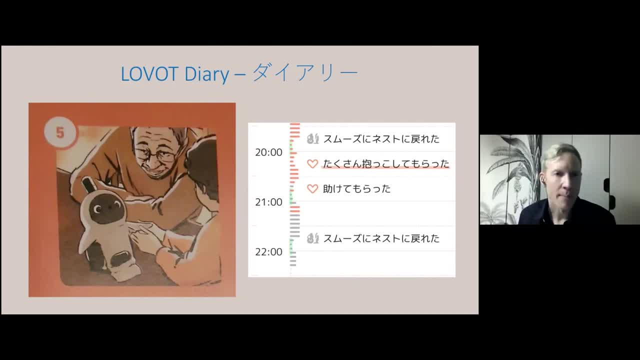 thinking about. you know emotions in a very much a rapid, ongoing, contextual and social and historical context. so what I want to emphasize here with this quick ethnographic vignette is that a market for companion robots in Japan is growing to meet what some producers think is a genuine desire to provide care and comfort- or iashi as it's known in Japanese- to people in 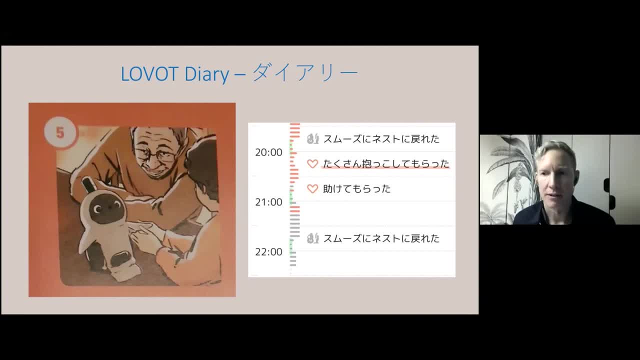 urban settings who are struggling to find it for a variety of reasons, and I think this point highlights the complexity of the technological, social and ethical problems facing the practice of building machines with emotional capacities. it also highlights why we want to make efforts to establish this dialogue across disciplines and how we might go about doing that in ways that can. 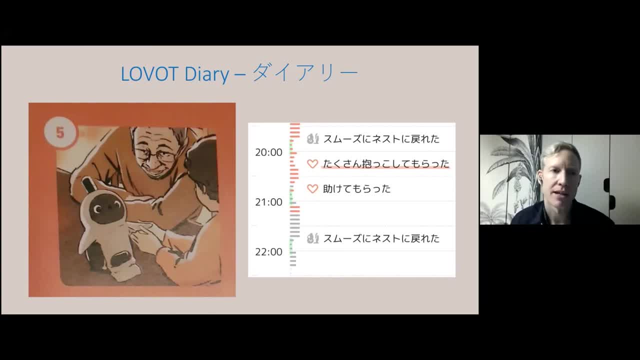 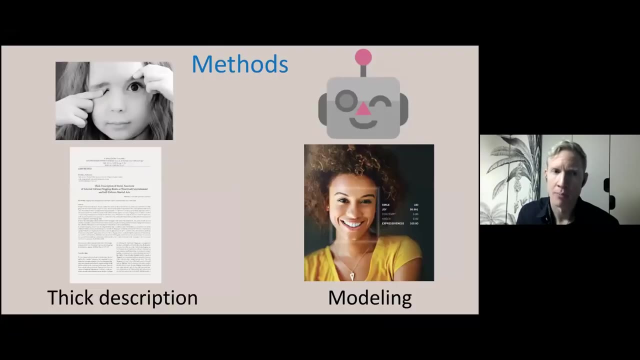 expand our vision of how emotional attachments are built into a variety of of systems or methods within that can serve a dev, a diversity of contacts, basically. so back to this problem of of dialogue and how both anthropologists or social scientists and engineers can approach this sort of coding, decoding problem. 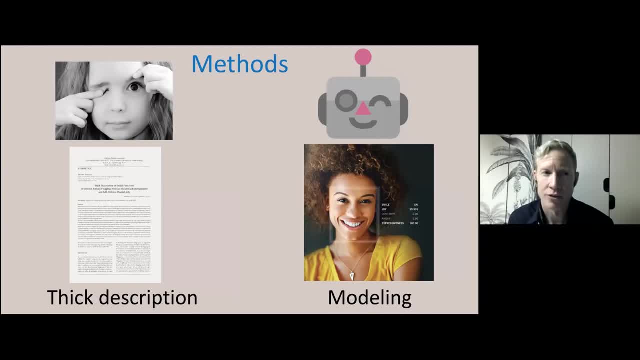 specifically complex emotions, like eye's reaction to a new artificial agent. so the fact that different approaches to what emotions are and how they work by engineers and social scientists are characterized sometimes in these polarizing and different disciplinary terms seems to me to be an obvious problem, but it's also, I think, a problem that invites explicit 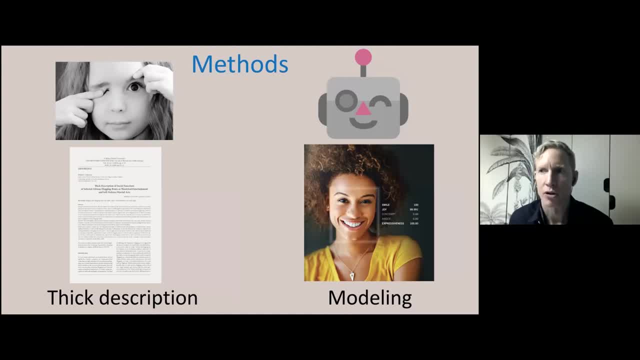 effort to address, in order to create these platforms and channels for cross or interdisciplinary dialogue and collaboration, something I'm sure most of you are are actively engaged in- and it's also an opportunity to, I think, explore ways of framing projects that can, precisely in order to facilitate collaboration, identify some common questions of common concerns. 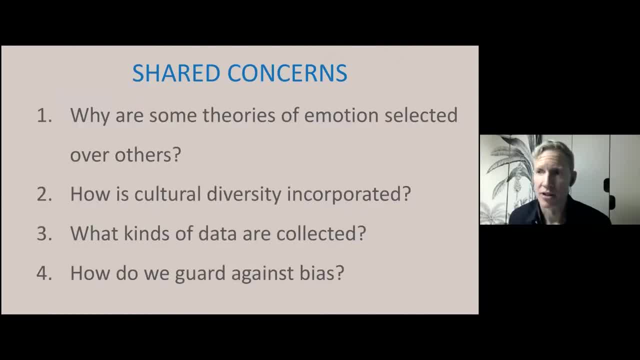 such as: what are some theories? why are some theories of emotions selected over others? And I tried to give a sense of this at the beginning of the talk. Also, how is cultural diversity being incorporated or left out of these models? What kinds of data are being collected? 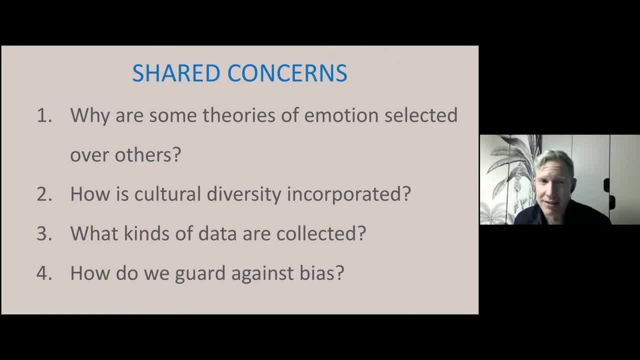 And I try to show a little bit of that with Lovat's diary there and his or her or its censors. And then, of course, how do we guard against bias? So these are all interests I think that all invested parties share and they can serve as starting points for experimenting, like robot engineers themselves do, with platforms for interaction and sometimes for collaboration. 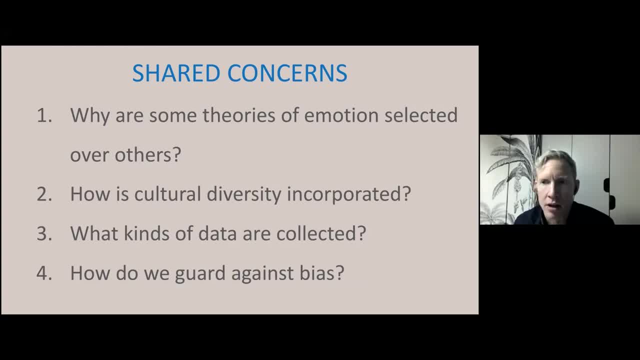 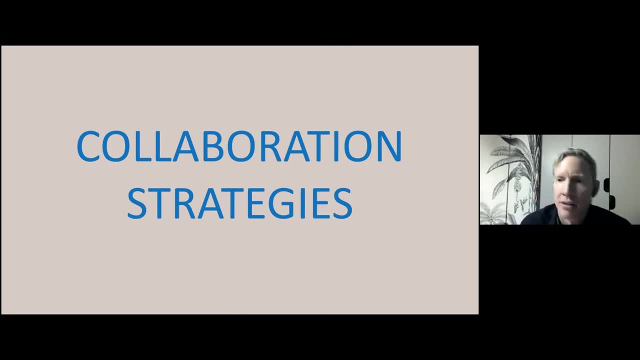 And this has been one major feature of our own projects- model emotion. So I want to talk briefly about how we aim to build dialogue between us as anthropologists, anthropologists and scientists, And then talking with engineers, And because I think this is where we can likely have the most productive discussion, I'll just briefly summarize a few things we do here and then I'll try to turn it back to our host and to the audience to facilitate our discussion. 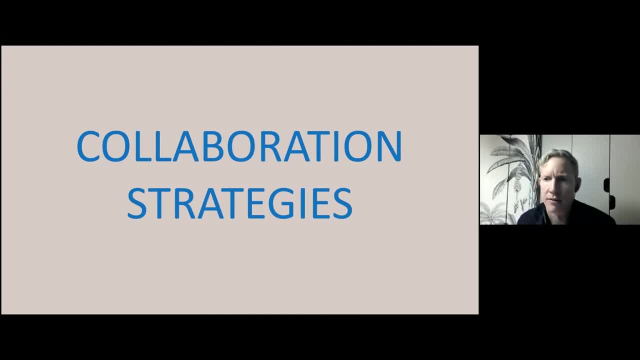 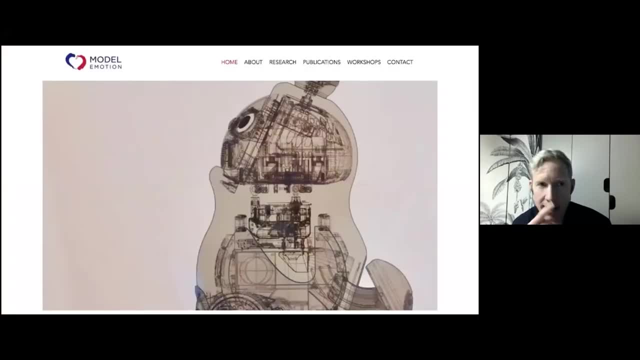 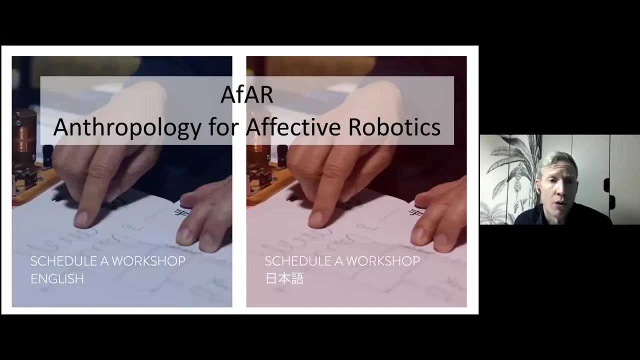 But let me briefly just highlight a few things that we do. The first and kind of the most predictable thing we do is obviously construct our website, which we do, We use as a platform for not only communicating our research but also connecting with engineers and and constructing the main feature of what we do in field work, which our workshops essentially, which we called anthropology for effective robotics. 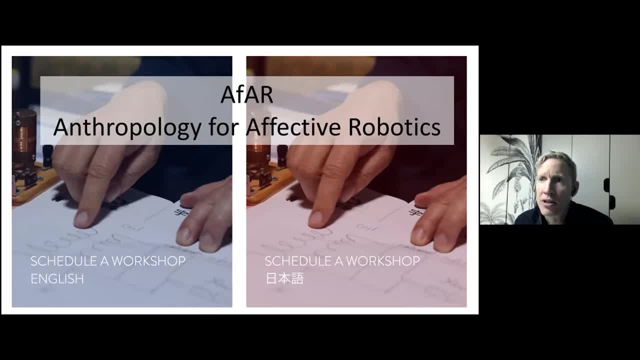 And what we do here in these robots is is basically offered to conduct these, these workshops at laboratories. We have done research on the vois and the. we have done research on the vois and the, And so in many contexts where we propose to exchange approaches to emotions from our perspective as anthropologists, that perhaps engineers might take some interest in, 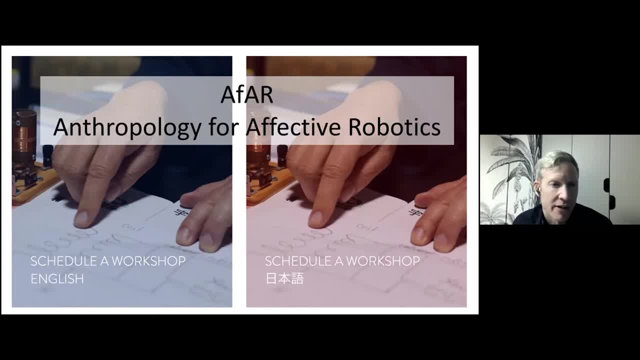 And we also, as anthropologists, try to generally genuinely learn from engineers how their own methods are technological tools for recording emotion. We as anthropologists- we as anthropologists- might not have considered So. it's absolutely this. the aim of these workshops is to construct this two-way communication, this two-way channel for communication. 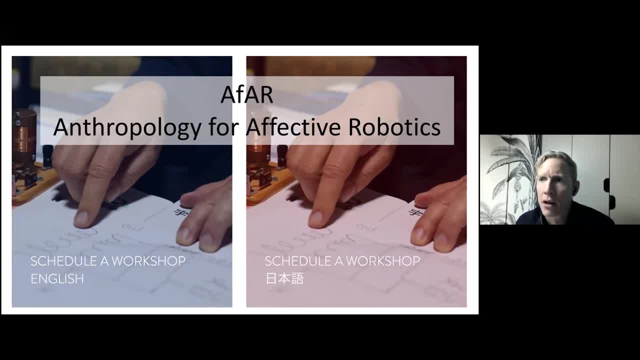 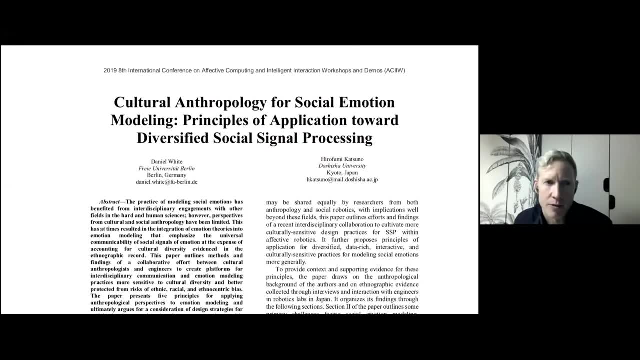 and generally learn from each other. So another strategy we use is to- I mean, obviously write not just for anthropologists but actually experiment writing as anthropologists but for engineers. So this paper was written for the major international effective computing conference in Cambridge and was given to those engineers who are specifically building machine models for 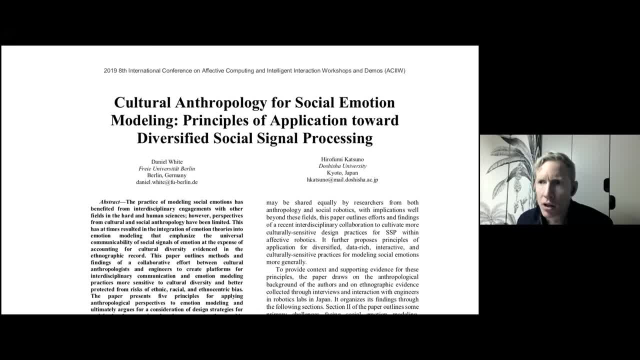 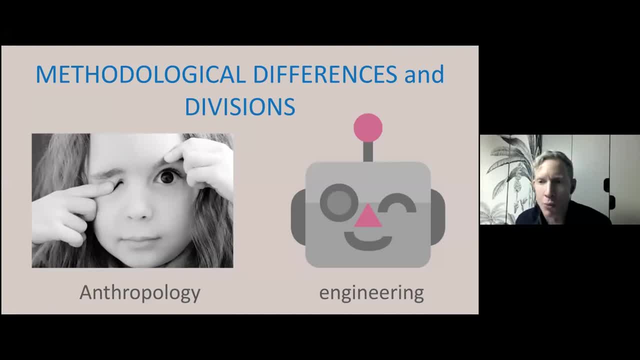 emotion detection And in this paper we tried to highlight what we saw as a common aim for engineers and anthropologists- And you'll see why in a minute, why I keep showing these images of winking or blinking- And that was to use basically this common aim that. 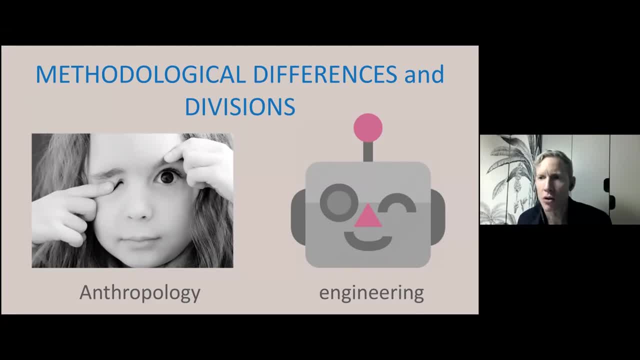 that we're trying to achieve And that was to use basically this common aim. that that we're trying to achieve And that was to use basically this common aim that that we see as engineers and anthropologists having, is to basically use all the tools at our 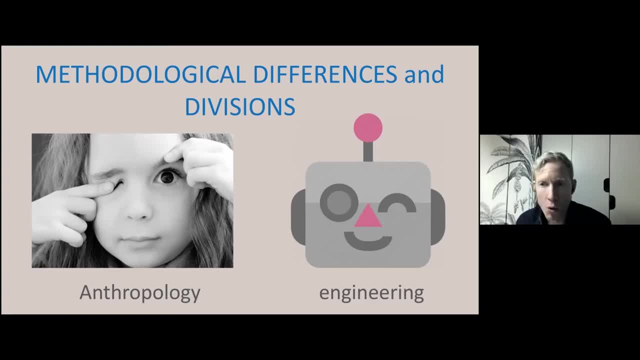 disposal- interpretive, quantitative, qualitative or otherwise- to catalog the incredible social diversity and granularity of human emotional responses and experiences. And we often do this by using a classic example from anthropology, from Clifford Geertz, about what it means to interpret the meaning of somebody winking at another person. And Clifford Geertz asks- and I'll: 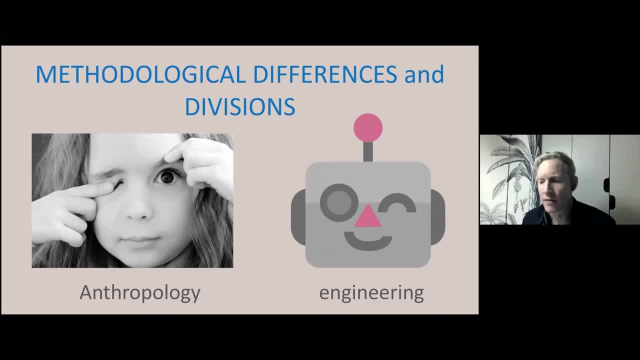 you know what's the difference between the sort of involuntary contraction of an eye versus what we might call a wink, versus what we might call a deceptive or sarcastic wink, versus what we might look at someone rehearsing a sarcastic wink in the mirror to be performed later. 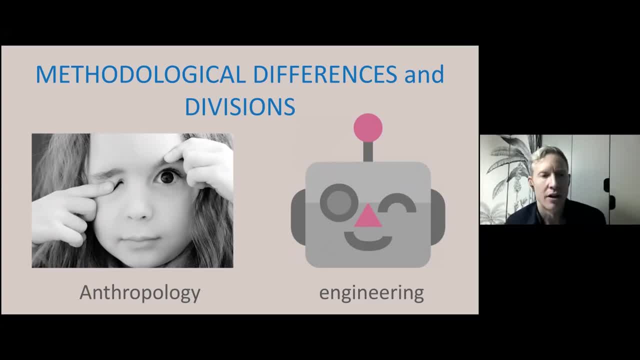 How do we understand all those different valences or those different meanings of what a wink is and how would an engineering perspective approach that and what are some of the limitations in that, in both of those perspectives, that we can use as a starting point for conversation about how to think beyond these differences between quantitative and qualitative methods. 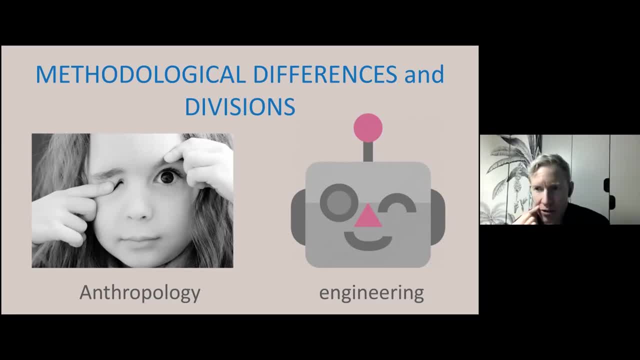 We also highlight in this paper, which is written very much to the best of our ability in a language common to engineering, a set of five principles that we thought engineers could apply and practices of building what they call social signaling models, in order to understand the meaning of what a wink is. 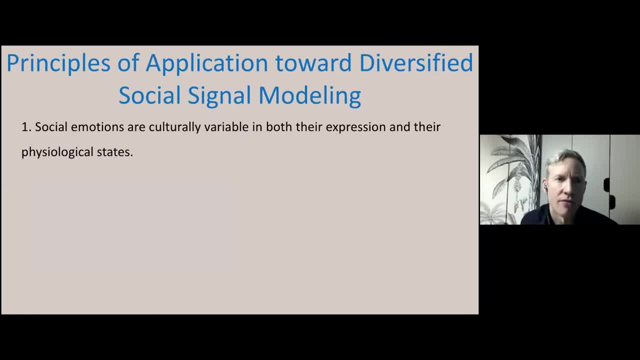 So I will leave that to Clifford. So in the building we can see that there are four principles, one of which is that it's about being a positive and positive person, but also about being a positive person, both of which are interested in being a positive person, andrà. 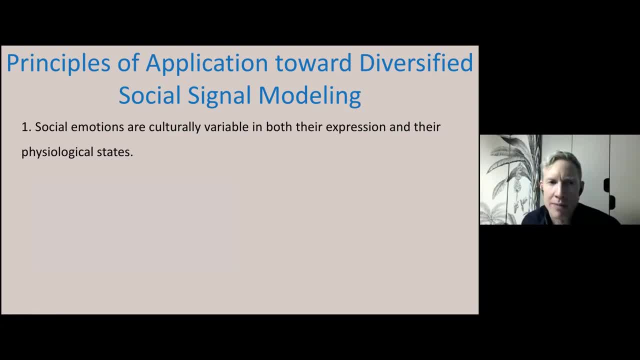 ev get a better understanding. So another example which has been really more for our and not for cultural diversity in their models. So we offer some principles, like- and this is not something that the получ would very often do, We would often like to speak in principles for ourselves. 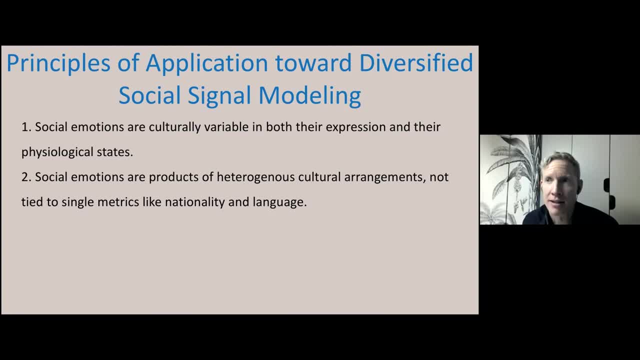 products of heterogeneous cultural arrangements which are not tied to single metrics like nationality and language, which is often how culture- quote unquote- gets constructed in laboratories. Social emotions are indexical, they're dynamic. I can go into that later if you're interested, but I'll just kind of keep those keywords up on the screen for now. 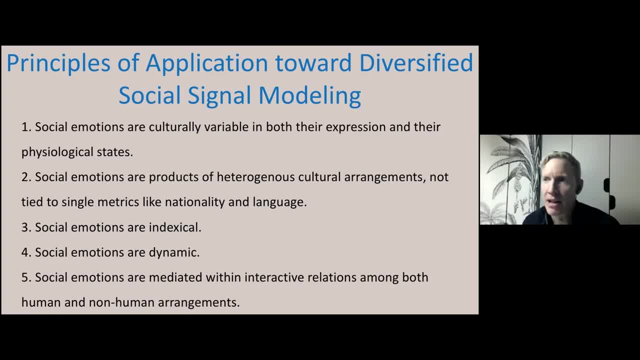 And social emotions are mediated within interactive relations among both human and non-human agents. People react in emotional ways to artifacts and objects, as well as to other beings. Obviously, this is a big interest in building evocative-like machines for specific reasons, And I'll even say: 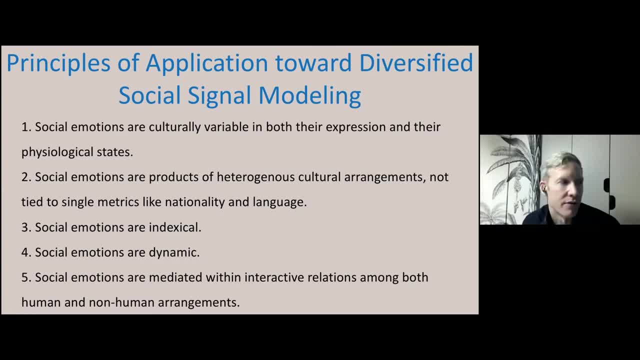 that you know, for anthropologists to use the word social emotion is a bit redundant for us because we would see all emotions as having this emotional and indeed this historical component. And even though we get the social component quite often in engineering laboratories, we often miss this historical aspect to what an emotion is. And I